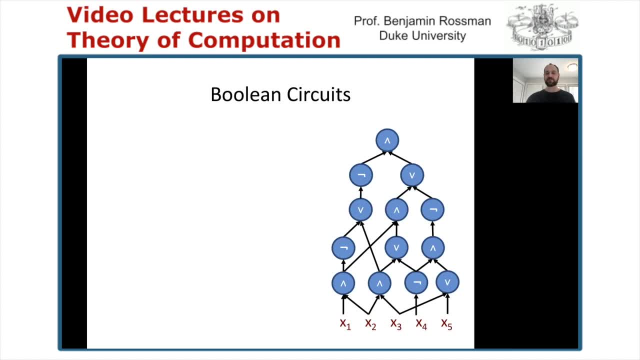 So the model of computation that we study for computing Boolean functions are Boolean circuits. So you see here, a circuit depicted on the right circuit is comprised of and or or not gates, and the inputs are just the coordinates of the string. So the way we would formally define a Boolean circuit. 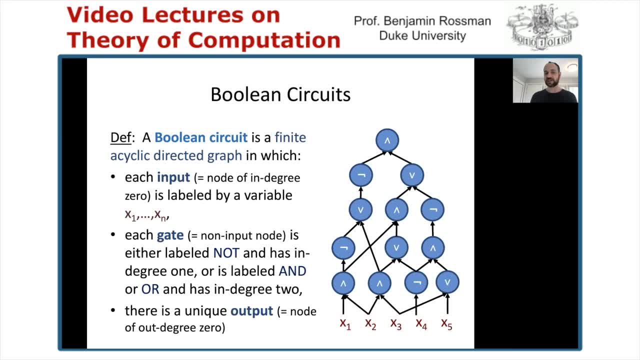 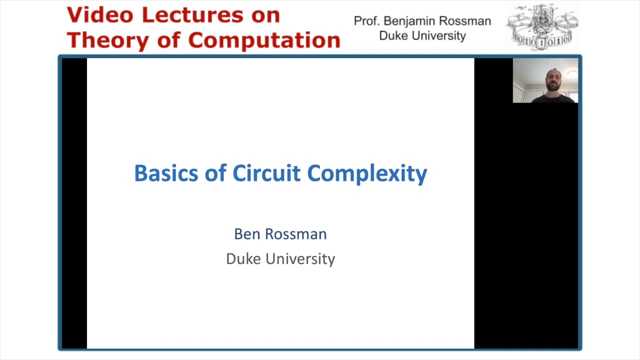 is as follows: so as a finite acyclic directed graph in which each input is labeled by a variable train of Bob. they're not- and let me start over because this sucks, sucks- basics of circuit complexity. so the central objects of study in circuit complexity are boolean functions and boolean. 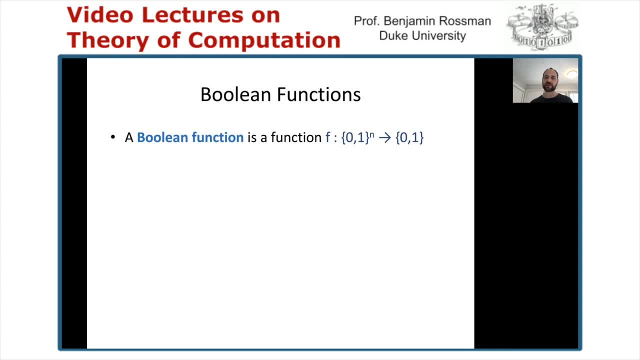 circuits. a boolean function is a function from the hypercube, so the set of n-bit strings to zero one, and a running example in this lecture will be the n-bit parity function, denoted x or sub n. this maps a string x to the parity of the number of ones in x, so the sum of coordinates x1 to xn modulo 2.. 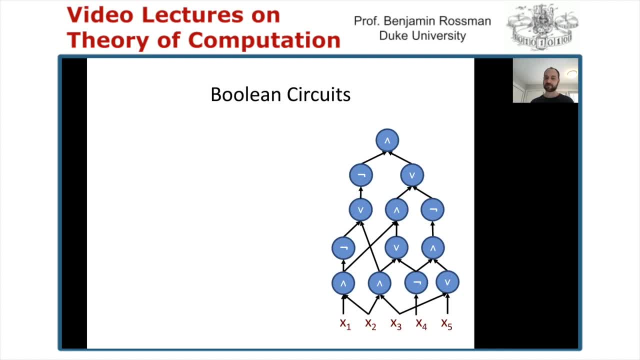 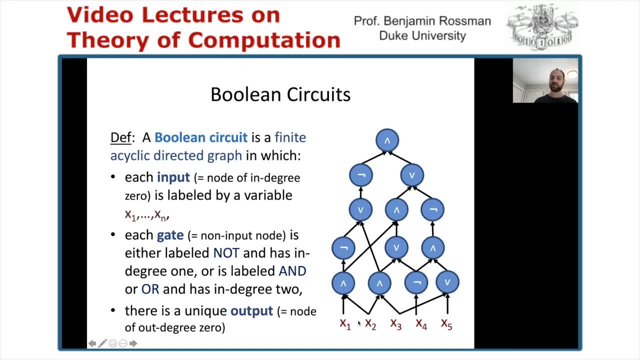 whose inputs are labeled by the- the coordinates of the input string, and each gate in the circuit is either a- not gate within degree one, or an, and or an or gate within degree two, and there's a unique output gate at the top which is producing the function. 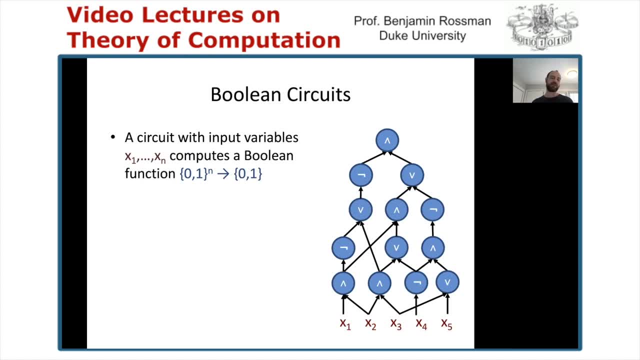 that the circuit computes. so a circuit with n input variables computes a boolean function of n variables in the natural way, and the two parameters we'll consider of boolean circuits are the size and depth. so size we measure by the number of gates and the depth is the maximum. 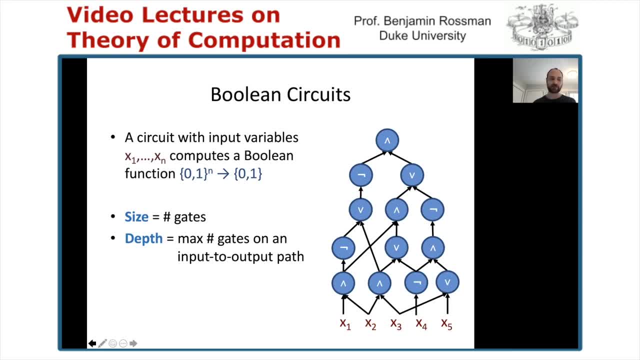 number of gates on an input to output path. so, for example, this circuit here has depth five. and just as a note, sometimes we measure size and depth only in terms of and and or gates. sometimes it's convenient to to ignore, not gates, in other words, let them count for free, okay. so this: 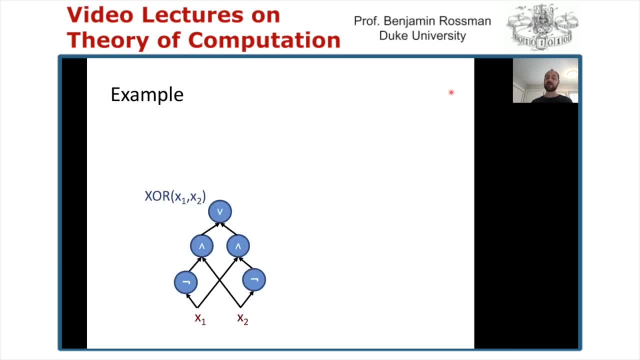 is the boolean circuits, computing boolean functions. let's look at some examples. so let's start with the two-bit parity function, in other words the exclusive or function on two bits. we can compute this as follows: so this circuit says either a x1 is zero and x2 is one. 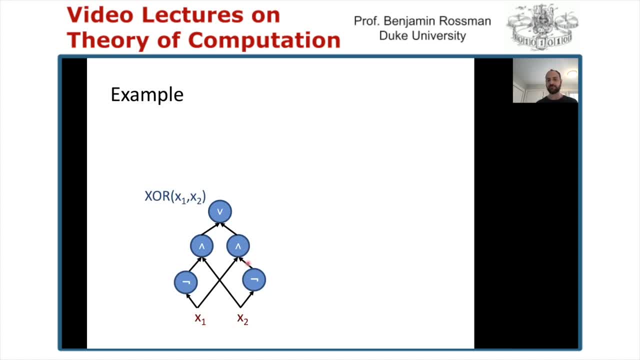 or x1 is one and x2 is zero. So this is clearly computing the exclusive or of x1 and x2.. Let's say we wanted to build the four bit parity function. Well then, we could make a separate copy of this circuit. 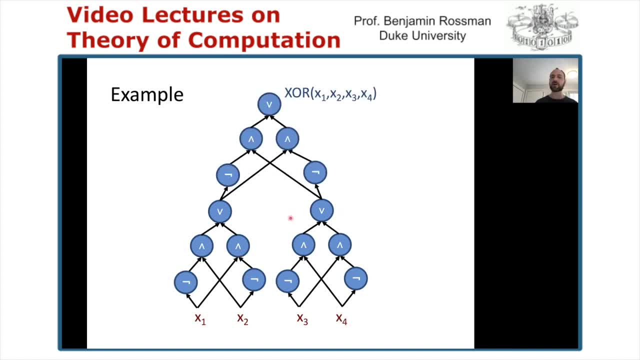 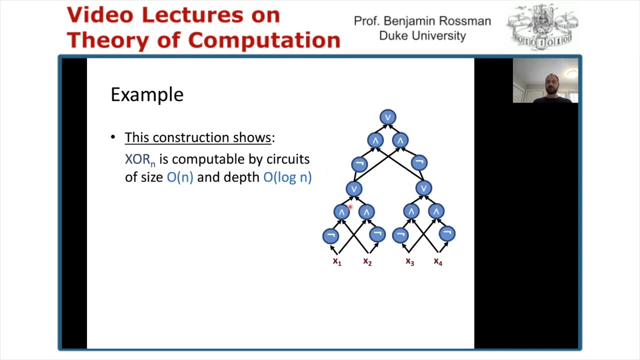 over x3 and x4, and then another copy on top, taking these two XORs as inputs, And in this way we get a circuit computing the four bit parity function. Okay, we can generalize this construction to any n and we get circuits computing parity of size, order n. 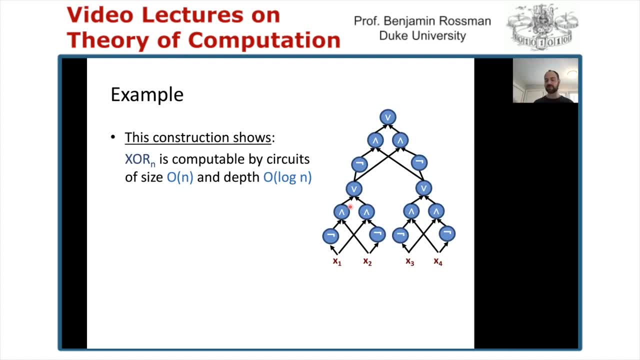 and depth would be order log n. if you build these circuits up in a balanced way- And in fact you can check for yourself that in total you'll get three n minus three and and OR gates and depth, two log n plus order one. 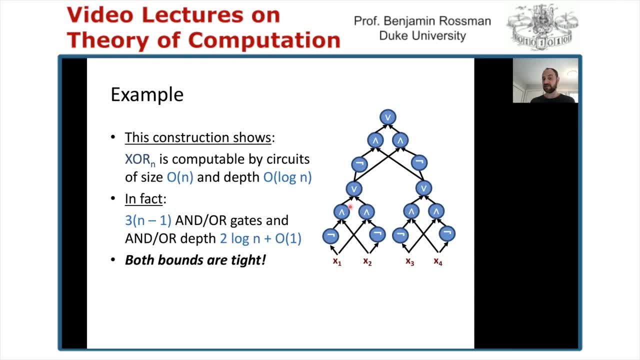 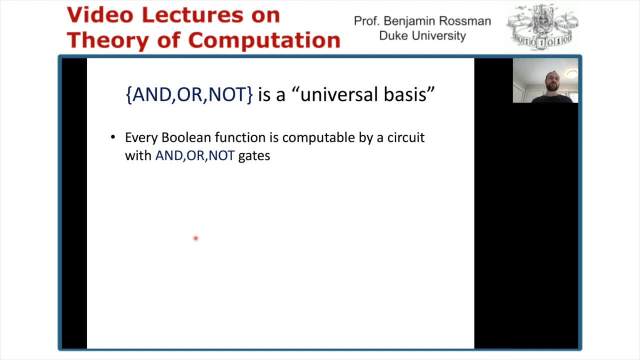 And it turns out you can show that both bounds are tight, and we'll actually discuss this later on. Okay, so, and or not? it turns out that it's not true. It turns out you can compute any Boolean function with just these three gates. 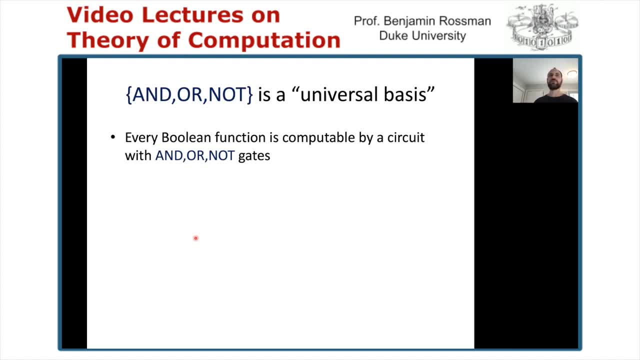 And so we say that the set and or not is a universal basis. So the term basis refers to the set of functions that are available as gates in a circuit. So, as an exercise, you can convince yourself that even if we just have and and not gates, 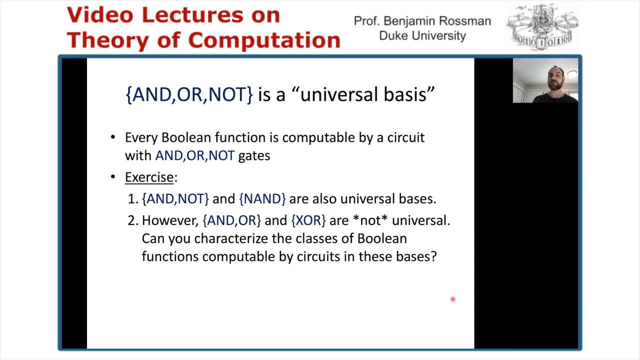 so if we don't have OR gates, then still we can compute all Boolean functions. This is essentially follows from De Morgan's law that expresses OR in terms of and and not. Even if we just have a single binary NAND gate, computing the not and function on two variables. 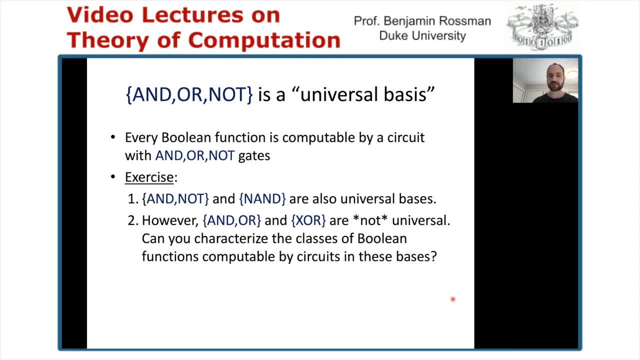 that by itself is a universal basis. Two non-examples are just the set of and and OR gates. So if I don't allow you negations, that's known as the monotone basis And just a single binary XOR gate is also not a universal basis. 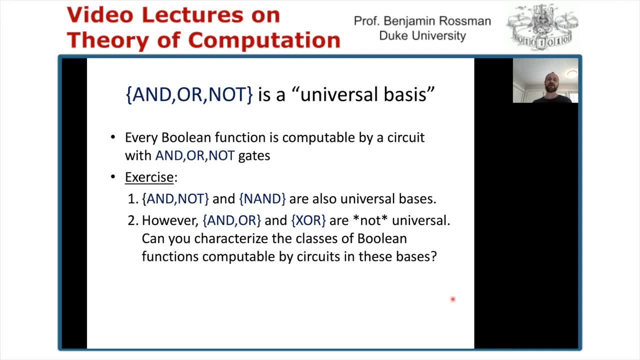 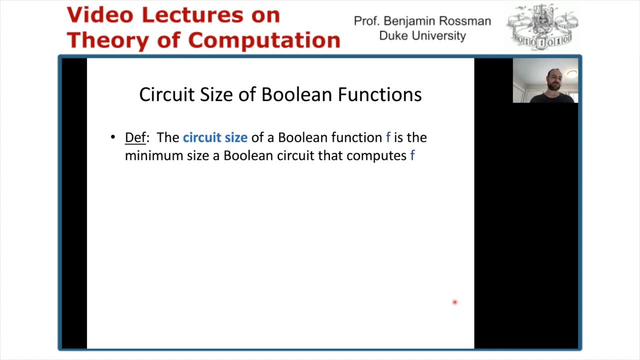 And it's a good exercise perhaps, if you haven't seen this before, to characterize the classes of Boolean functions that are computable by circuits in these bases. Okay, so Boolean circuits give us a way of measuring the complexity of Boolean functions. You could measure this by size or depth. 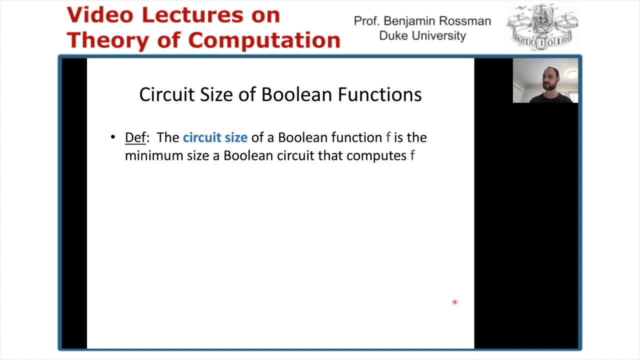 but here's the definition of the circuit size of Boolean function. This just refers to the minimum size of any Boolean circuit that computes that function And This is up to constant factor. This is notion of circuit size, is sort of independent of the choice. 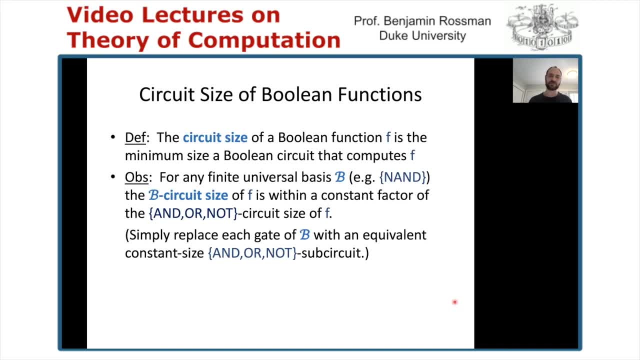 of a finite universal basis. So the observation is that for any finite universal bases b so set of possible항 gates, мои possible gates, the b circuit size of f is within a constant factor of its boolean circuit size. and 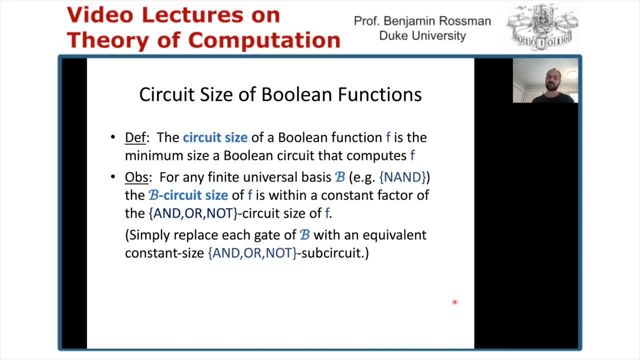 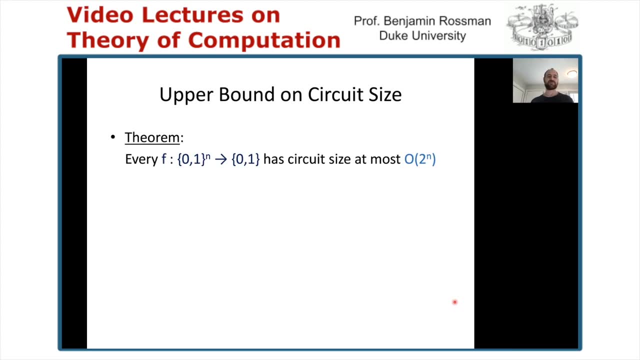 to see this. you would simply replace each gate of the basis b with an equivalent constant size boolean subcircuit. okay, so let's, uh, let's uh, make a quantitative version of this claim that every boolean function is computable by a boolean circuit. so, in fact, we'll. 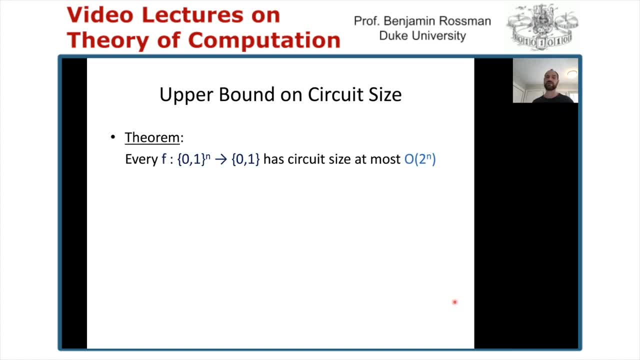 show that an n-variable boolean function is computable by a circuit of size at most order 2 to the n. okay, so let's see how, how we can show this. so it's going to be a proof- by induction on n. so consider the two n minus 1 variable boolean functions, f0 and f1, where f. 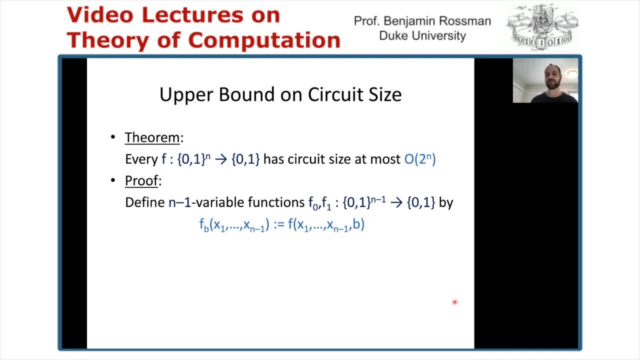 sub b is obtained by nella sub c minus one f0 to the n cube of function by substituting the constant B for the variable XN. And we're going to define in a circuit C sub F computing F as follows. So assume we have circuits CF zero and CF one. 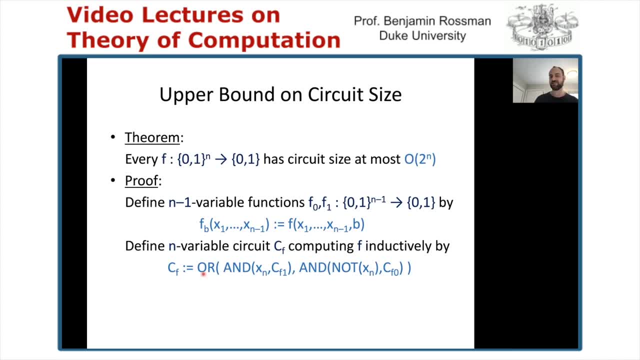 then C of F will be the circuit as follows. We're saying either XN is one and CF one is one or not XN. so XN is zero and CF zero is one. Okay, so if you just think for a moment, 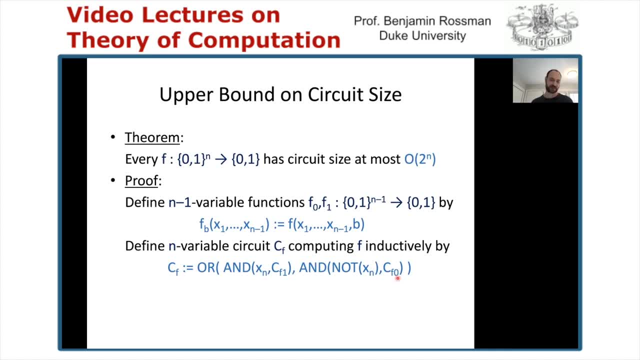 you see that this circuit, indeed, defines the function, computes the function F And, clearly, the number of gates in the circuit C sub F is: well, we have all. we have the gates from CF one, we have the gates coming from the sub circuit CF zero. 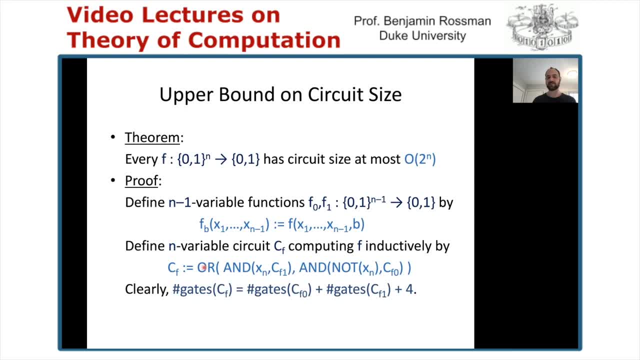 And then in addition we have four extra gates. this or and and and not. Okay, and then by induction it follows that the number of gates in CF F will actually equal this number here, which is order two to the N. 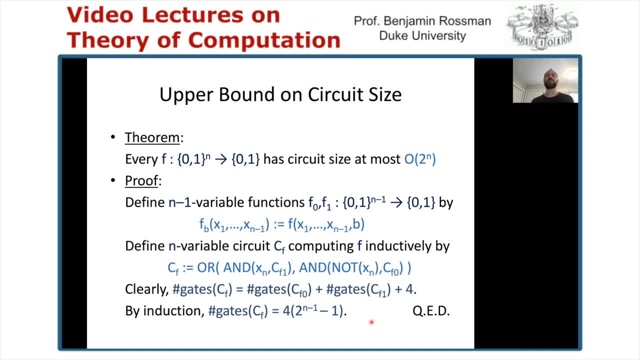 Okay, so this is one way of showing that every Boolean function has at most exponential. so meaning that every Boolean function has at most exponential. Okay, so this is one way of showing that every Boolean function has at most exponential circuit size. and, uh, this, actually a stronger upper bound is known. it was shown by lupinov, i believe in. 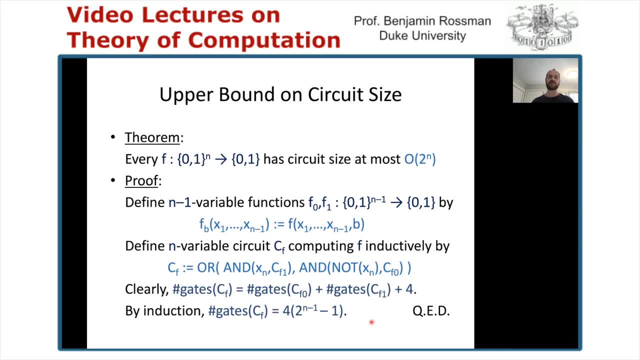 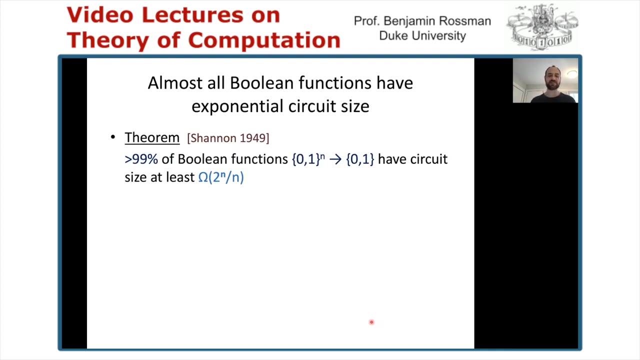 58, 1958, that uh, you can actually uh construct circuits of size order two to the n divided by n, so slightly smaller, and that's that's uh, uh, by a more more clever construction and that turns out to be tight. okay, so we're next going to see one of the earliest results in circuit complexity. 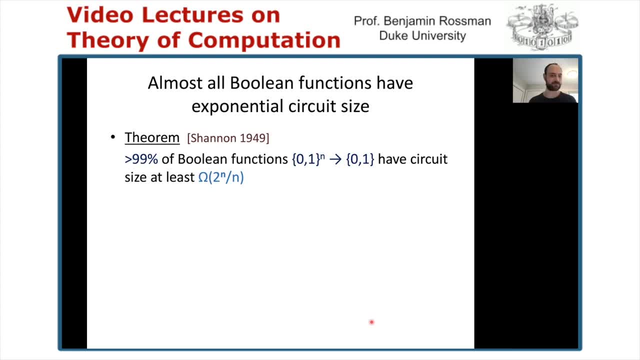 proved by claude shannon in 1949. okay so almost all boolean functions and for concreteness let's just say more than 99 percent of boolean functions on n variables require exponential circuit size. in particular, have circuit size at least omega of two to the n over n. 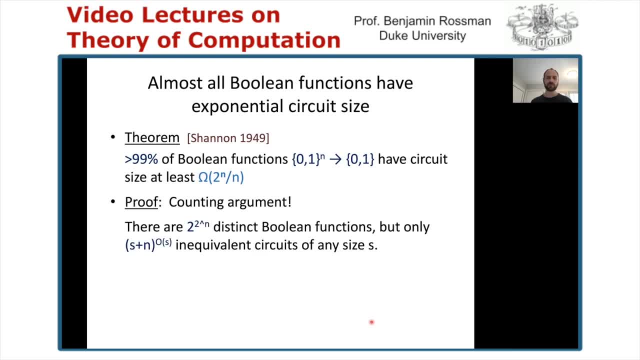 okay, and the proof is very simple. it really is. it's just a counting argument. so, on the one hand, there are two to the two to the n, uh, distinct boolean functions, and to see this, note that there are two to the n points in the hamming cube and to specify a boolean function, you just 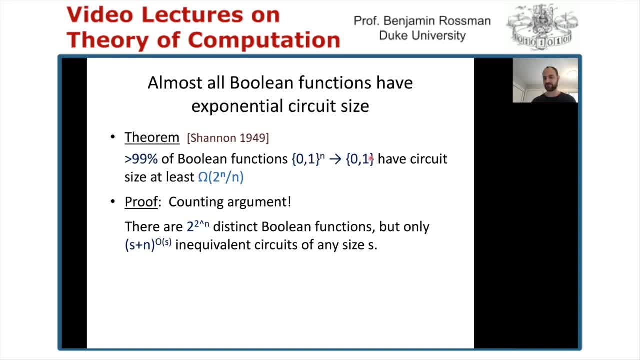 you, for each of those points in the hypercube you're assigning it zero or one. so there are exactly two to the two to the n distinct boolean functions and there are two to the two to the n overall boolean functions. but on the other hand, um, i claim that there are at most this number. 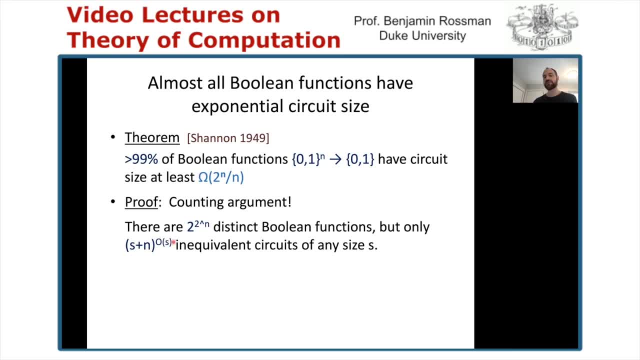 s plus n to the order s in equivalent circuits of any size s. so here we're really counting the number of distinct boolean functions that are computable by size s, and it's a easy exercise to show that you can bound this by by essentially s to the 2s. okay. 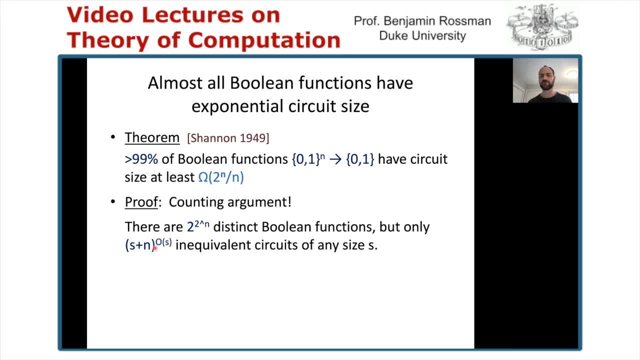 okay, the reason for two here is because for each and or or gate, you know it has wires to to two different sub-circuits. okay, so won't give the details of that argument. but once we have this, this claim, in hand, then the theorem follows immediately. it follows that, to compute even 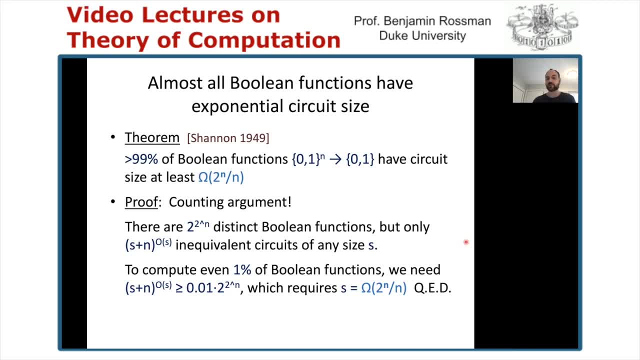 one percent of all boolean functions. well then, we require that that the number of equivalent circuits of of psi of the given size is at least one percent of two to the two to the n. so we would need this inequality, but this means that the size s has to be omega of two to the n. 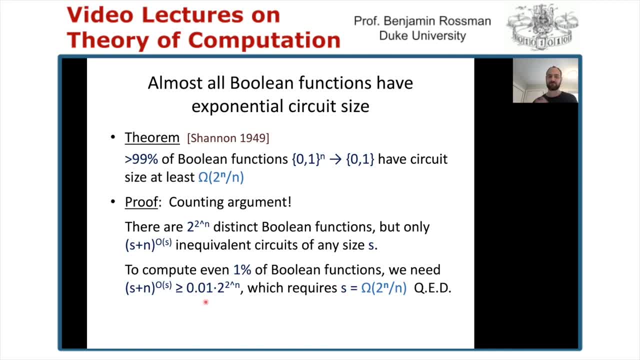 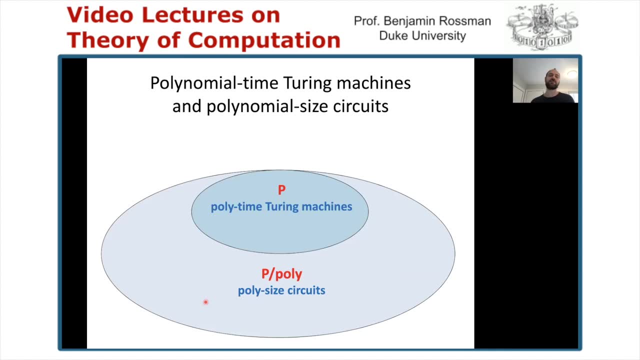 over n, right? so that's very simple proof which establishes that almost all boolean functions have exponential circuit circuit size. okay, next we're going to define a complexity class associated with circuits, so this is known as p slash poly. okay, so it's going to be. this is this. 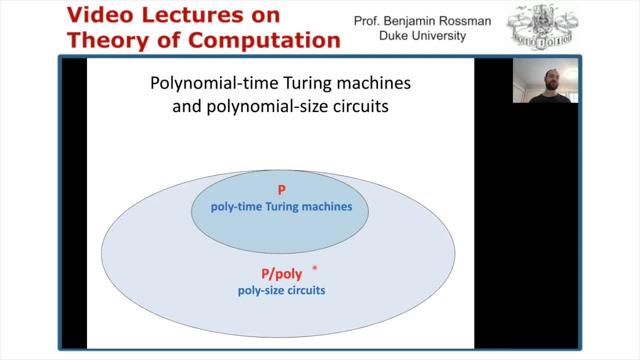 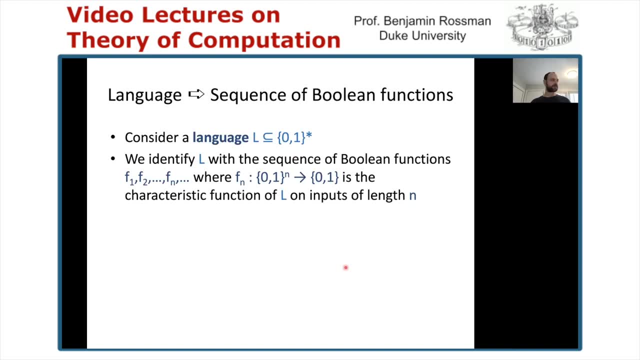 is the circuit, or so-called non-uniform version of p, as as i'll explain. so um so, so far in this, in this uh online lecture series, we've been studying the complexity of languages, right? so a language l is just a set of circuits that are associated with circuits, so this is the. 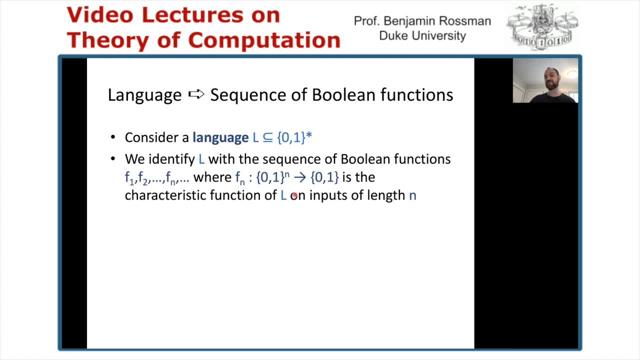 set of strings of arbitrary lengths, so zero. one to the n is zero, one star is just notation for string. you know all strings of zeros and ones. um, so we can identify a language, l, with a sequence of boolean functions. okay, namely the. the the nth function in the sequence is just a characteristic. 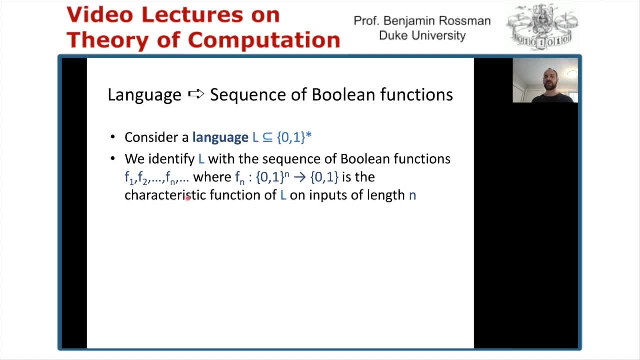 function of the language on inputs of length, n. right, so fn of x, in other words, equals one. if fn of x is equal to n, right, so fn of x is equal to one. if fn of x is equal to one, x is in the language L and zero. otherwise. 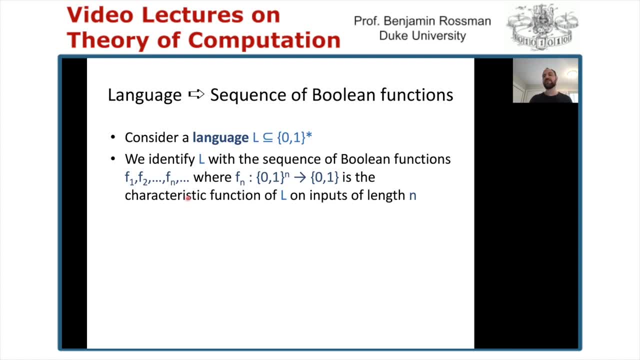 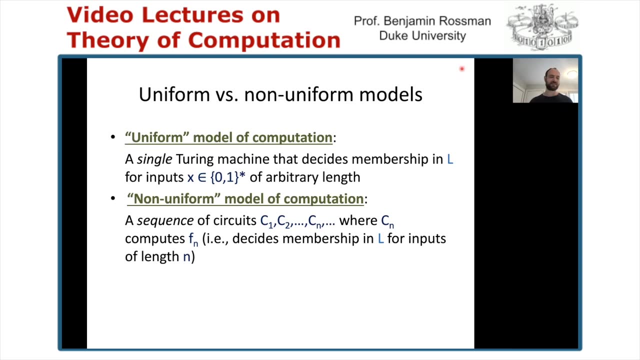 And this is a one-to-one correspondence between languages and sequences of Boolean functions. Okay, so this lets us study the complexity of a language in terms of circuits, And here there's an important distinction that we make in complexity theory between uniform and non-uniform models of computation. 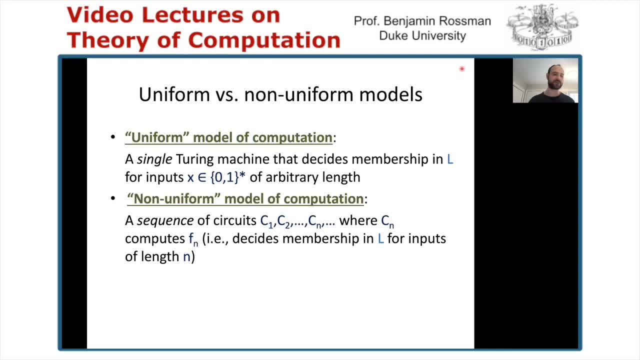 So so far you've encountered already various uniform models of computation, For instance a single Turing machine which decides membership in a language, L for inputs of arbitrary length. So if for any Turing machine you can run that Turing machine on inputs of any length, 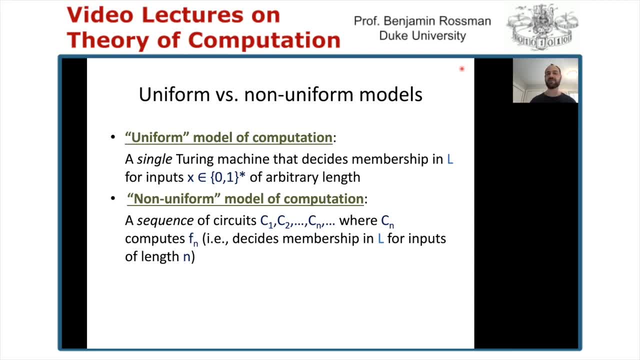 Similarly, a deterministic finite automaton would be another example of a uniform model of computation. Non-uniform refers to having a sequence of of models. you know circuits, say. you know one for each input length. So to compute a language, L, non-uniformly. 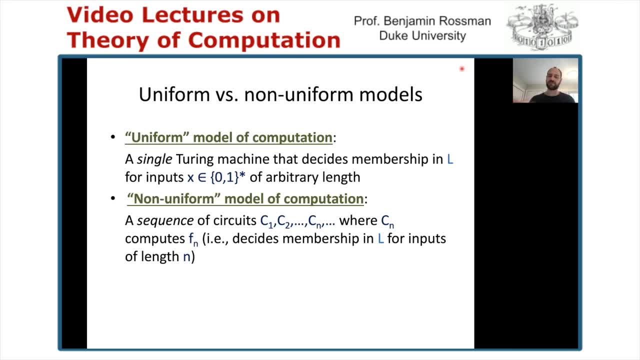 we have just a sequence of circuits where CN is deciding membership in the language, but only can be run on inputs of length N. So when we speak about algorithms in the traditional sense, usually we have in mind uniform models of computation, In particular in the uniform model, and you know. 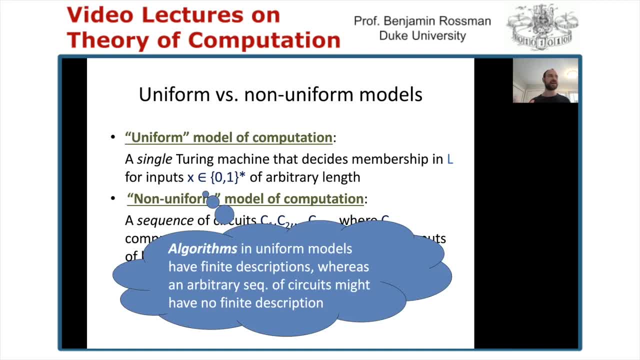 a single Turing machine or algorithm has a a finite description that you can write down. So, in contrast, an arbitrary sequence of circuits does not necessarily have any finite description. okay, So we don't make any assumption about how the sequence is being generated. Okay, so let's, let's just recall, uh, what we, what we're doing, is we take, uh, so let's, let's just recall, uh, what we're carrying out. And so we're taking this for a second right. 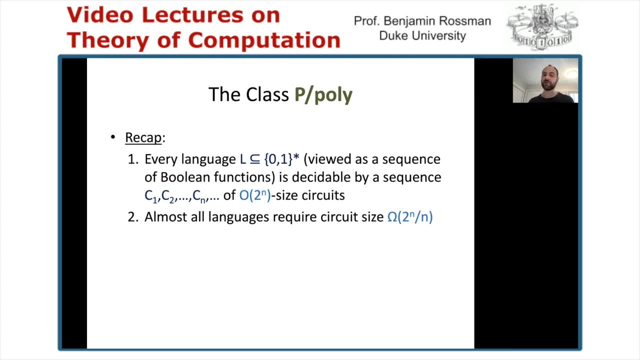 So that that's a little bit more complicated than the simple one, what we've shown so far about Boolean functions, but in terms of languages. So to recap what we showed earlier, every language L viewed as a sequence of Boolean functions, is decidable by some sequence of exponential size circuits. 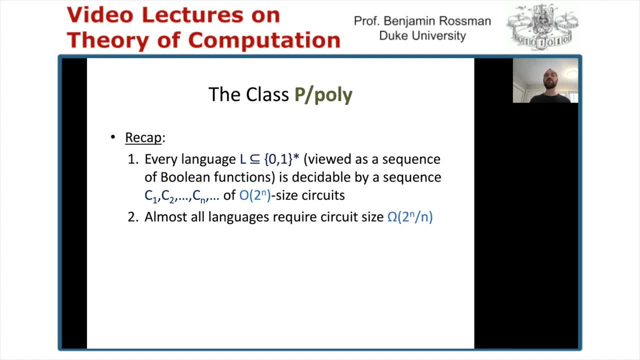 And then we showed Shannon's theorem that almost all languages, on the other hand, in fact require exponential circuit size. So this leads us to the definition of the class P slash poly. So this is the class of languages that are decidable by polynomial size circuits. 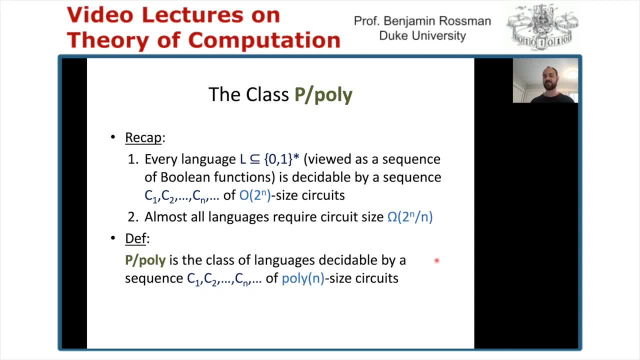 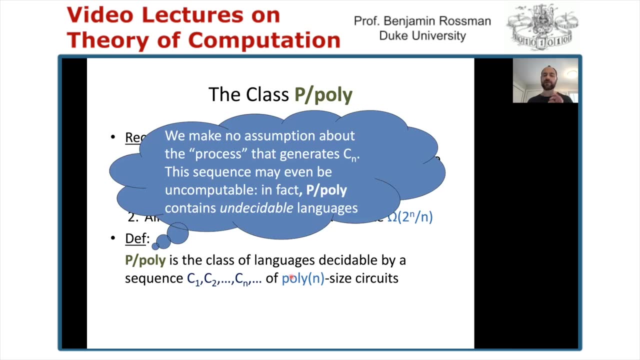 Okay, so much less than the worst possible exponential circuit size. Okay, so, in other words, languages with efficient circuits. So your, and just to reiterate the point, we make no assumption about the process that generates these circuits, CNN And, in fact, the sequence of circuits. 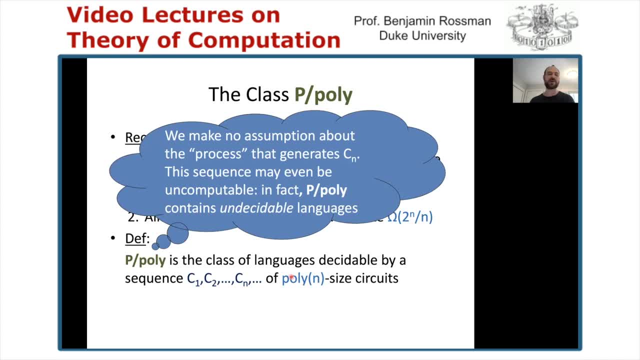 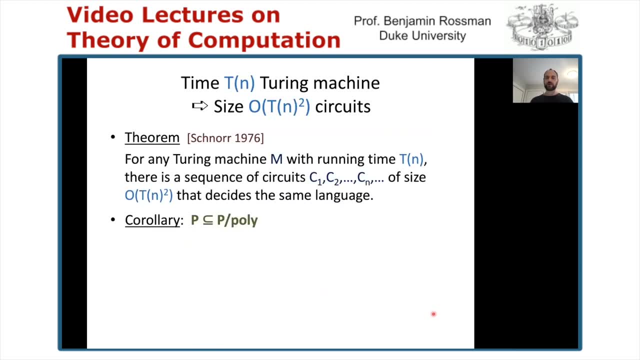 can even be on computable. moreover, P slash poly you can easily show even contains an undecidable languages. Okay, you could, you can sort of hardwire and undecidable language into the sequence of circuits. Okay, that p. so the class of polynomial time decidable languages is a subclass of p slash poly. 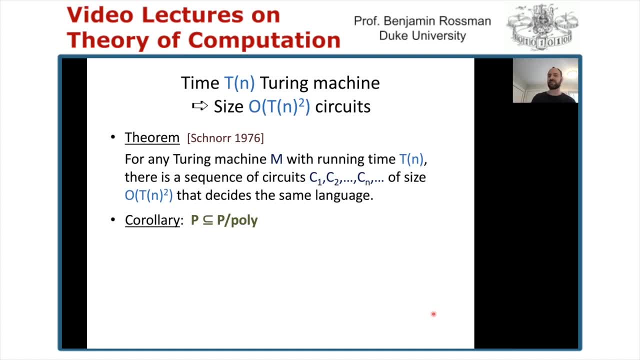 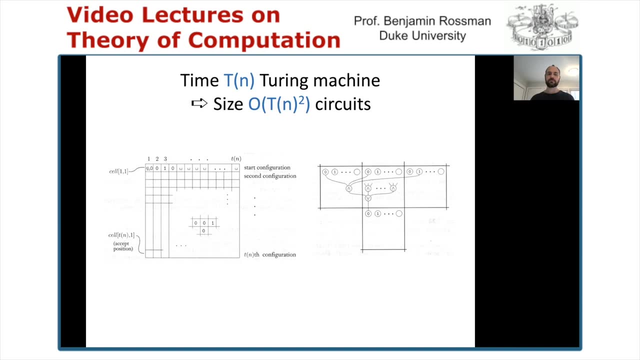 Okay, so the circuits are actually a more powerful generalization of Turing machines in some sense, And so this follows from the following theorem that any Turing machine m with running. Okay, here's an illustration of the construction, And these diagrams are copied from Sipser's book, So the idea is based on what's known as the tableau. 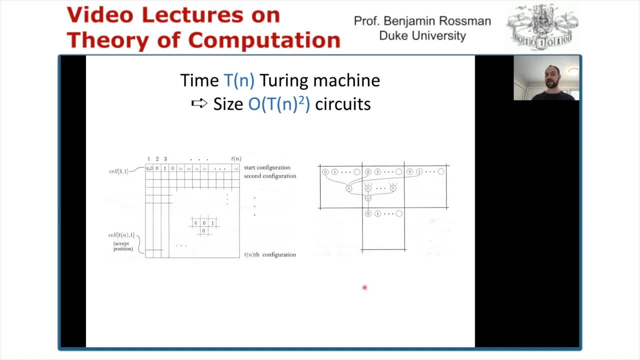 of the Turing machine m on a given input x. So this, the tableau over here on the left, is a table a, t by t table, and each row of the table contains a configured table And each row of the table contains a configuration of the Turing machine at the given time. 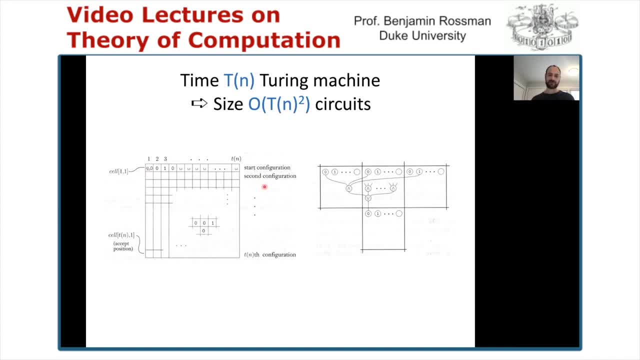 So on the top row is the initial configuration of the Turing machine, then the next row would be the configuration after one time step, and so on. So the configuration contains the contents of the tape, together with the location of the tape head and the current state. 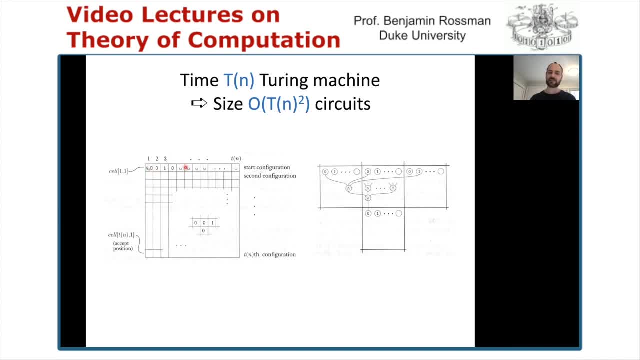 So initially the first n cells will contain the input x, followed by blank symbols Out to column t of n, And the first cell will contain also the state, the initial state, q0, indicating that the tape head is at the leftmost location in its initial state. 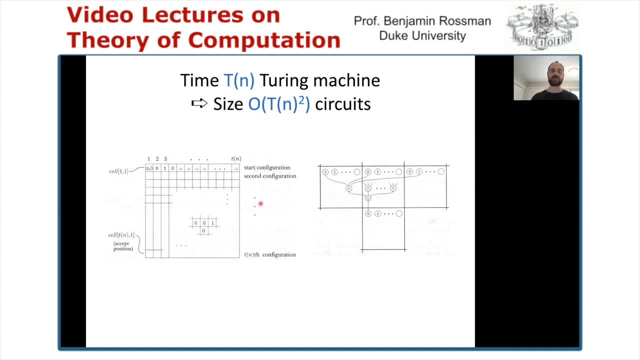 Okay, and so the you know. for example, if the first step of the Turing machine were to overwrite this with a one and then move to the move, the tape head to the right, then the next configuration would have one zero, one zero, And in the second cell we'd additionally have 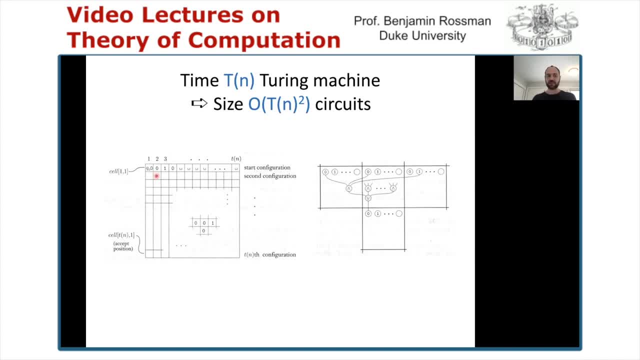 whatever the state is at that point Good, And we can assume, without loss of generality, that the Turing machine always halts with the head in the leftmost position. So, therefore, to determine whether or not the machine accepts, it suffices to look in the contents of the leftmost cell, you know, the bottom left cell. 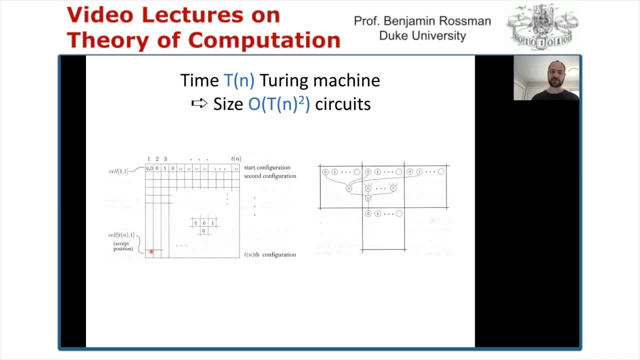 Now. so the idea of the circuits which simulate this tableau is as follows. So, each cell in the tableau, we can represent the information in that cell using a constant number of bits. Okay, so we'll have a constant number of gates which are which are computing the, you know, like a. 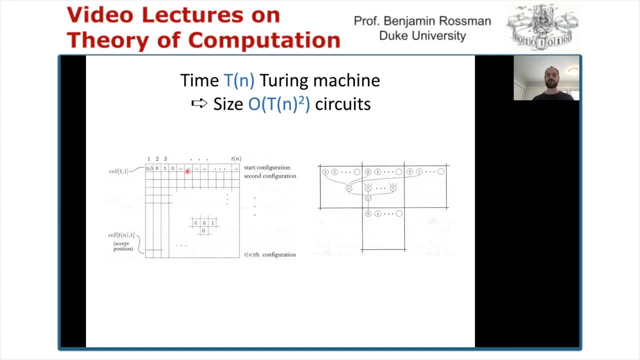 zero one representation of the tape, of the information in that cell. and so what is the information in that cell? we have the symbol of the tape alphabet, we have, you know, a bit indicating whether or not the tape head is at that location, and we have the current state of the Turing machine in the case that the head. 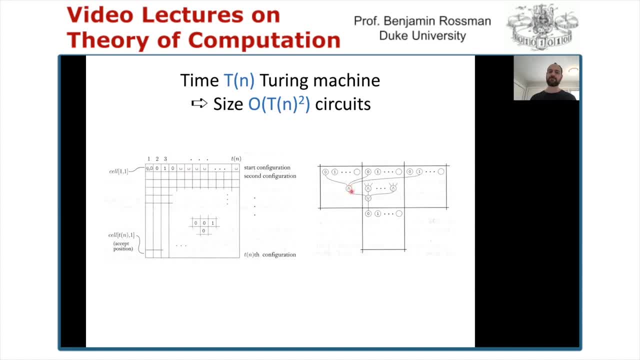 is at that location. so the observation is that, well, we only need a constant number of bits to represent that information. in particular, log of the size of the tape, alphabet plus log of the number of states is sufficient. and now, if we look at any cell in the tableau, so this cell here for 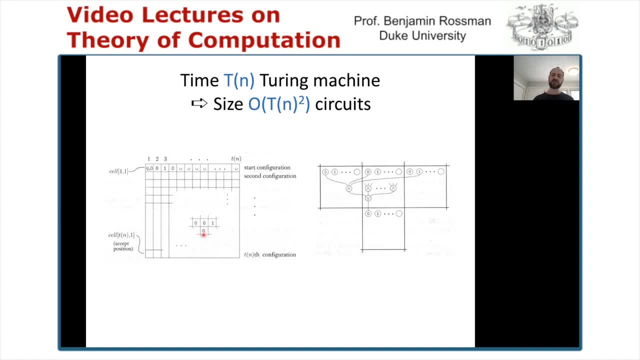 instance, we can observe that the contents of that cell are completely determined by the contents of the three cells above it right. so if the Turing machine head at the given at the previous time step is not in one of these three locations, then we know that we just copy for the entry above right and otherwise it's just a local. 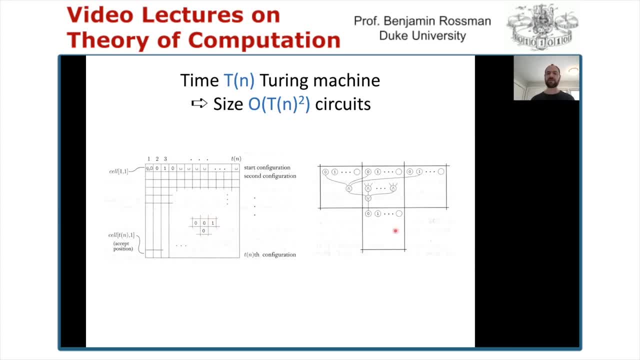 computation. and so in our circuit, you know, the circle will be divided into blocks corresponding to the cells of the tableau. maybe at the top you have the gates which are representing the actual data there and then to compute that data from the cells above, you can do this with constant size. 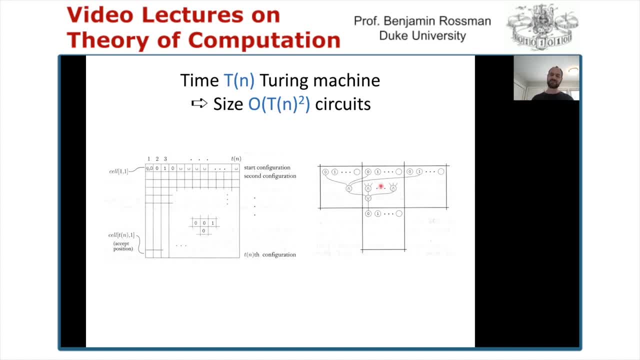 boolean circuits. and here I note that this in this circuit illustration, here the, the, the wires are being drawn like pointing downwards. in the rest of this lecture I'm drawing my circuits the other way, with wires pointing up. but anyway, you, you get the idea. so this is just a sketch of 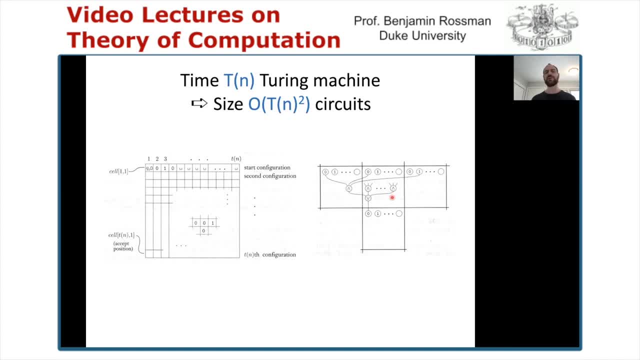 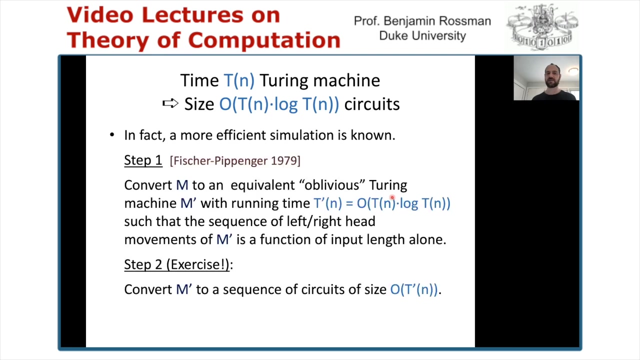 how this simulation works right, and we can see that the the size of the resulting circuits is T of m squared. I wanted to mention that a more efficient simulation is in fact known. so so there exists circuits of size T, log T, which simulate a time T Turing machine. so to just to outline, 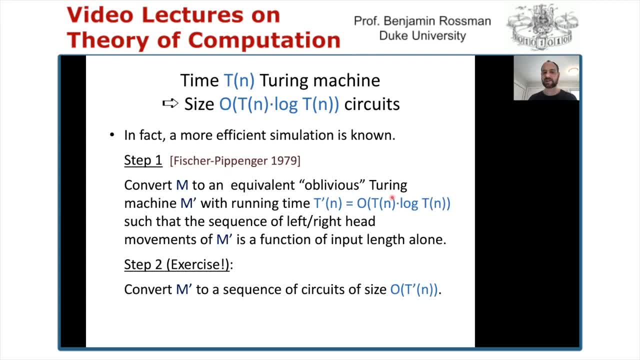 how that goes. so the first step is to convert any Turing machine m into what's known as an oblivious Turing machine: m prime with running prime, running time, t prime equals T log T, and oblivious means that the sequence of left to right head movements of m prime is a function of the input length alone. so on any two strings of the same length, the, if you. 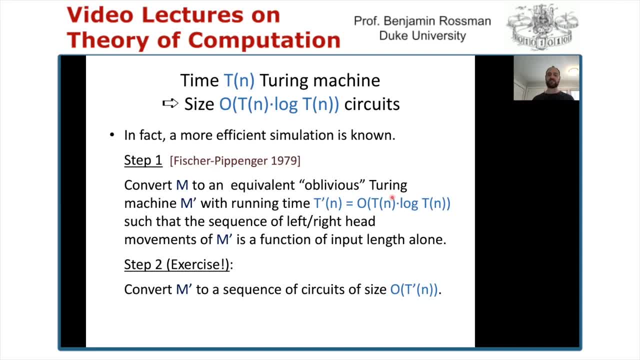 or if you're only looking at the sequence of head movements of m prime, they will be the same. okay, good, so let's take that, that step, for granted. that's a theorem of Fisher and Pippenger. then the second step, which I leave as an exercise, is to convert m prime. you know. 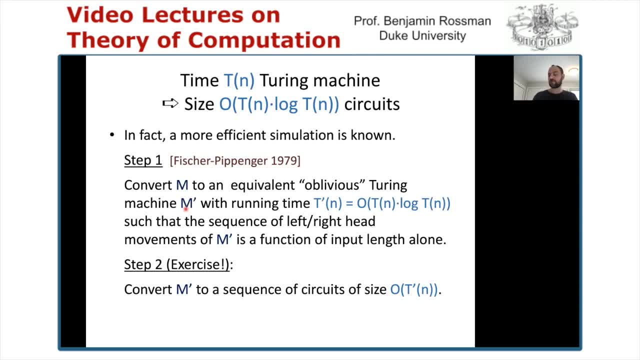 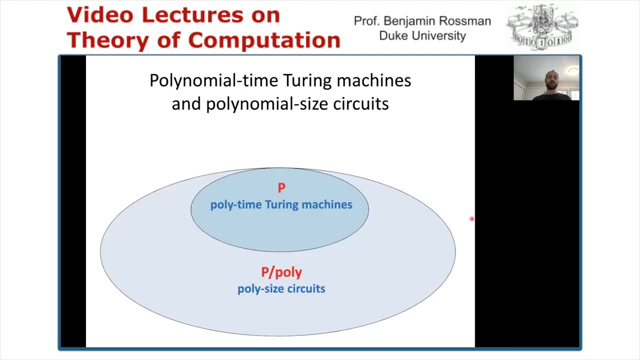 with the oblivious Turing machine m prime to a sequence of equivalent circuits of size order T prime. okay, so there's a. there's a linear size simulation of oblivious Turing machines. okay, good, so we've now defined the class P slash poly and we've proved that it contains the class. 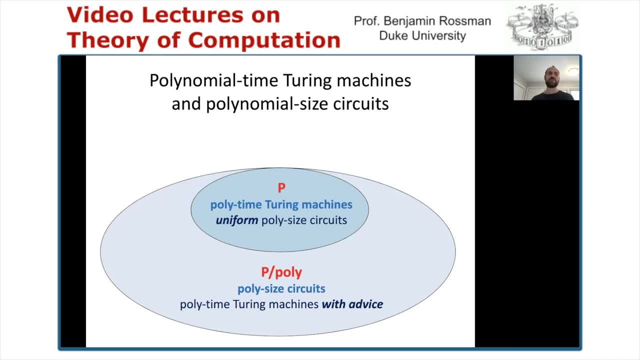 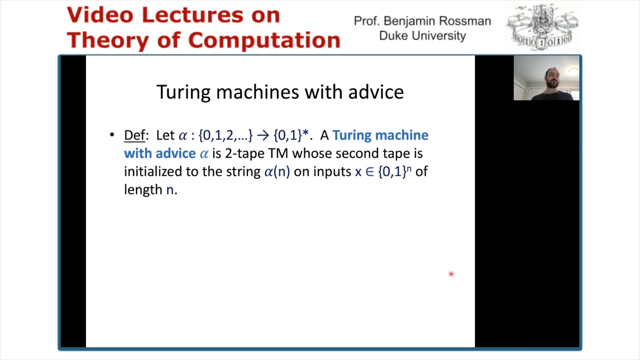 P. so next I'm going to describe alternative characterizations of both of these complexity classes. so both P and P slash poly can be characterized both in terms of Turing machines and in terms of circuits. so we'll think we'll define this one first. so okay, so this is the notion of a Turing machine with advice. so let alpha be. 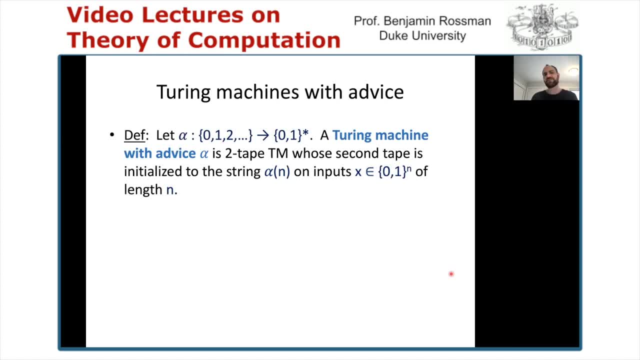 a function from natural numbers to strings. so we can also think of alpha as just a sequence of strings. so a Turing machine with advice. alpha is defined as a two tape Turing machine with one standard, you know input work tape and the second tape which is initialized to the string alpha n on inputs of length n. okay, so this is a Turing machine with advice. 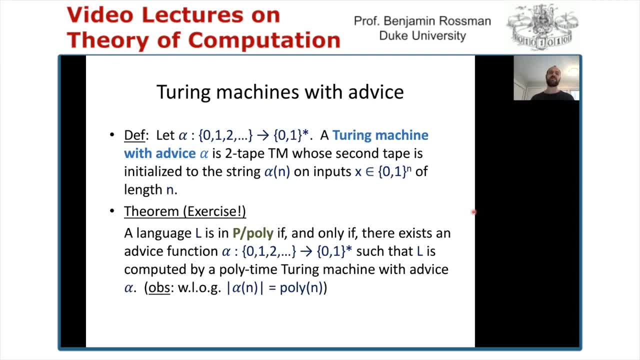 and so the. the theorem is that a language is in P slash poly if, and only if, there exists an advice function such that l is computed on all inputs by a Turing machine with advice alpha. and just a remark here that without loss of generality we can assume that alpha has polynomial length. 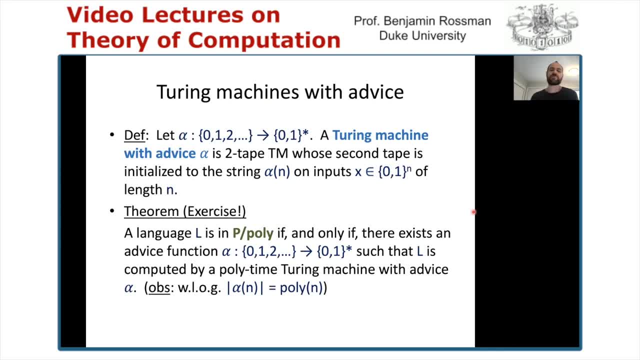 alpha n has length poly n, simply because a poly type Turing machine can only access poly n. bits of the advice term. okay and um, right, so I'll leave. I'll leave the proof of this as a, as an exercise. and uh did want to mention that this is, uh, the, the standard definition, in fact, of P slash poly. 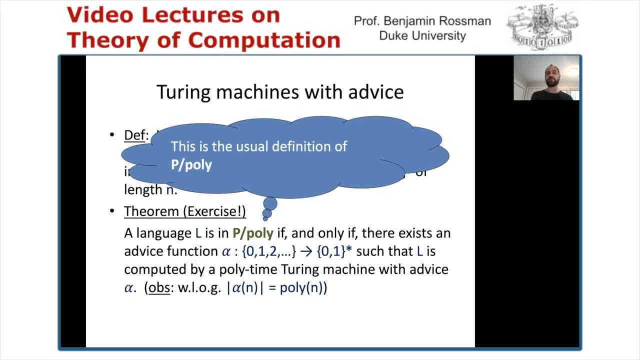 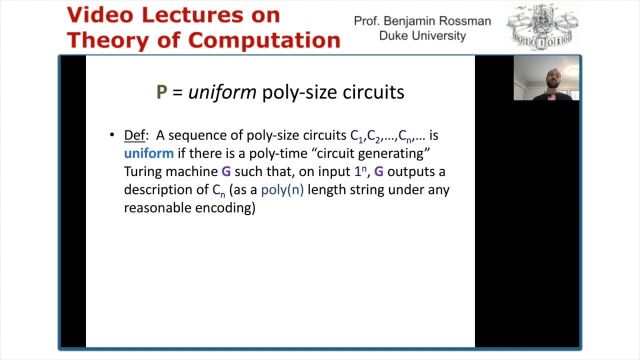 um. so this theorem is really showing that this definition is equivalent to the one we gave in terms of poly size circuits. good, so that we can also characterize the class p, so poly time languages, in terms of circuits, and this is via the notion of uniform circuits. so here's the definition. we say that a sequence of polynomial size circuits is 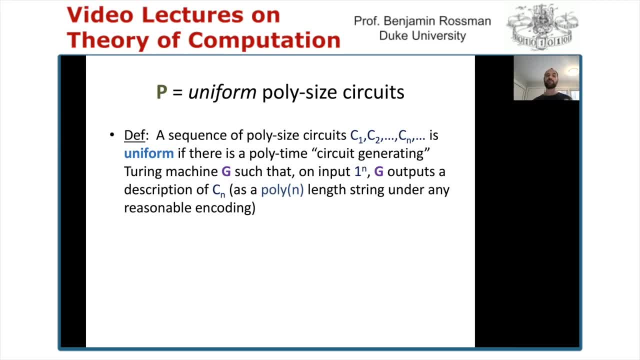 uniform if there exists a polynomial time Turing machine. g, so a circuit generating Turing machine such that on input one to the n entirely, u is a single string of length, N, so a string of ones of length n. g outputs a description of the nth circuit. okay, so description as some poly length string under any reasonable encoding. okay, so this is the. 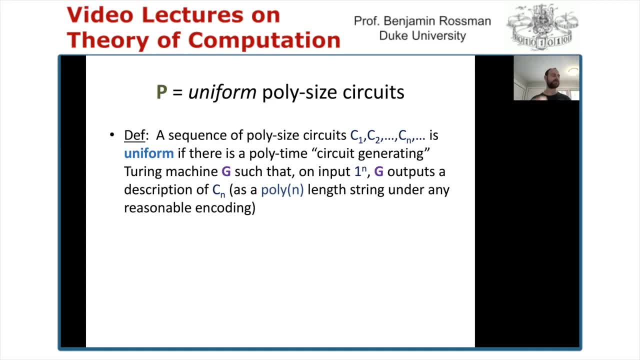 notion of uniform. so so earlier we were saying: you know, in the definition of p poly, the sequence could these circuits? Okay, and then? so the theorem is that a language is in P if, and only if, it's recognized by a uniform sequence of poli-sci circuits. So the proof of this. so one direction. 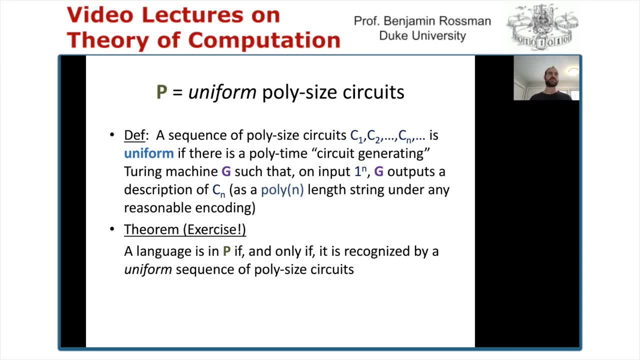 we essentially already saw the proof of. if you just consider this simulation of a time t Turing machine by circuits of size t squared, well, we'll see. you see that that is in fact a uniform sequence of circuits, That process we described. you can regard that as a poli-time. 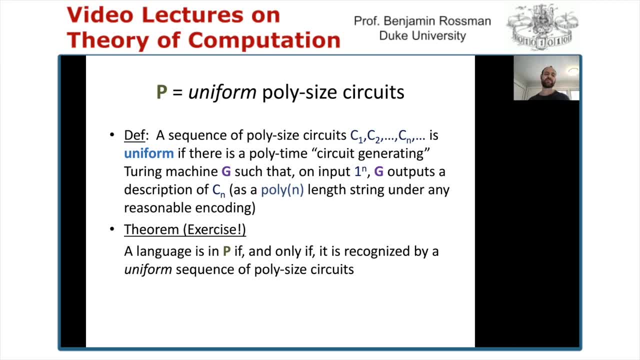 algorithm In the opposite direction. suppose we have a uniform sequence of poli-sci circuits generated by some Turing machine G. then we get a poli-time language by on input x. we first run the machine G on P and then we get a poli-time language on P, and then we get a poli-time. 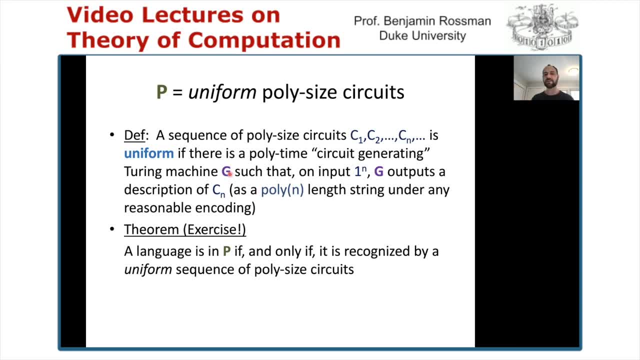 language on one to the N, where N is the length of x. This produces some circuits, CN, and then we simulate that circuit, which can be done by also by a poli-time Turing machine. Each of these steps is polynomial time, So this produces a poli-time algorithm for our language. And just to mention, 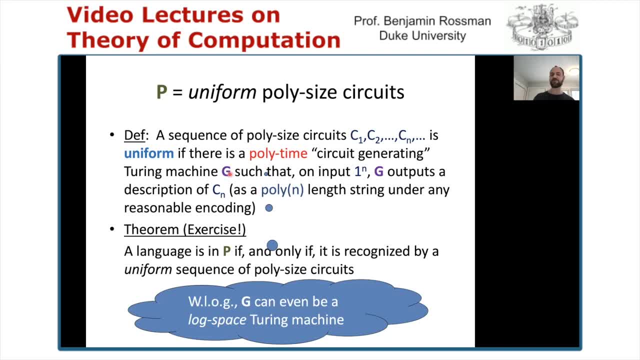 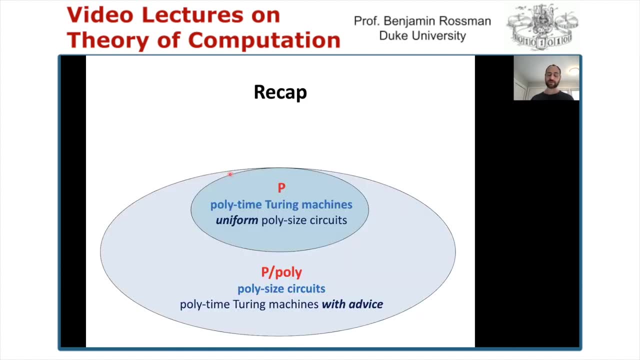 that there's even weaker notions of uniformity which lead to the equivalent definition of P, slash poli, sorry- of P. So you can even take G to be a log space Turing machine. So this is known as log space uniformity. Okay, so to recap, we've now seen definitions of both P and 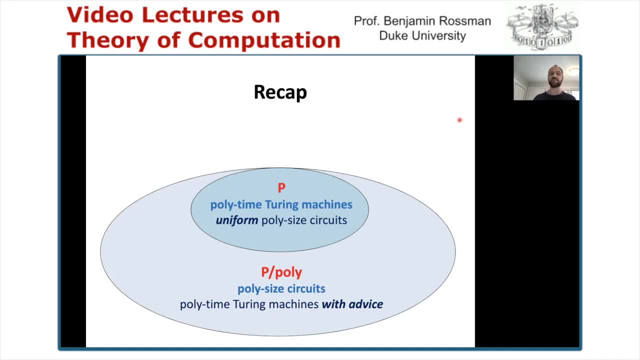 P slash poli in terms of Turing machines and circuits. And yeah, so we've seen that P is a subclass of P slash poli. So the question arises: where does NP fit into this picture? So well, of course NP can WiFi. on the other hand, it does not contain P slash. 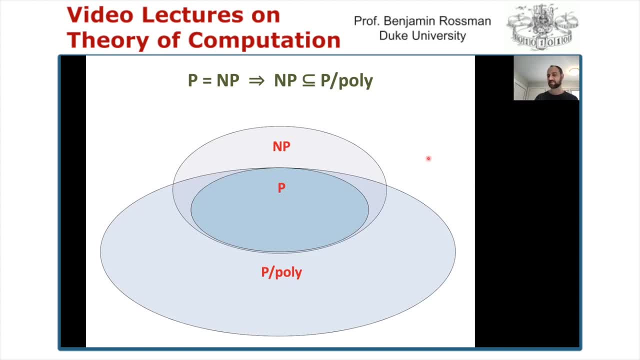 poli. So, as mentioned earlier, P slash poli even contains undecidable languages, whereas certainly every language in P or NP is decidable. That's one way of showing it. You can also argue that P and NP are countable languages. 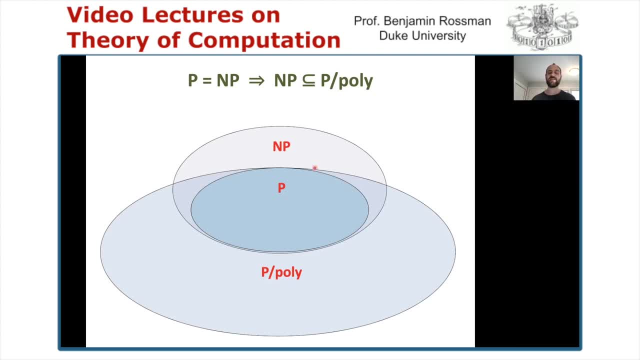 P and NP are countable languages. languages they're countably infinite, as are the class of decidable languages, whereas the class P slash poly is uncountable. OK, what about? so we know that P slash poly is not contained? 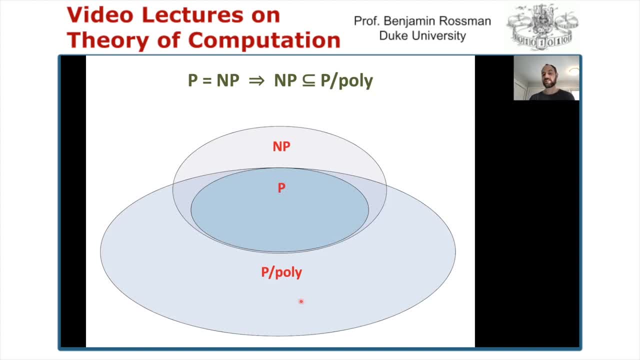 in NP. but what about the converse? Is NP a subclass of P slash poly? Well, we can observe that if P equals NP, then indeed NP is a subclass of P slash poly, And the contrapositive is that if NP is not, 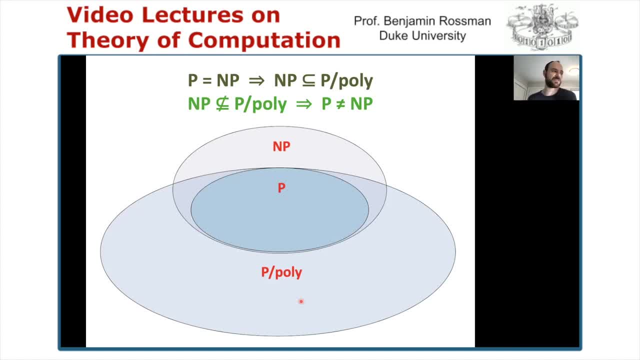 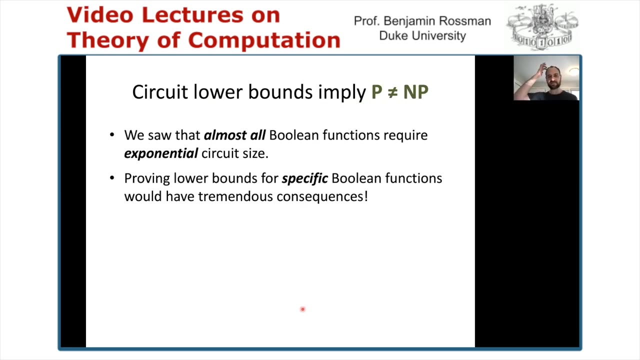 contained in P slash poly. So in other words, if NP languages do not have poly-sized circuits, then P is different from NP. OK, so this leads to the observation that circuit lower bounds Are a concrete combinatorial way of potentially separating. 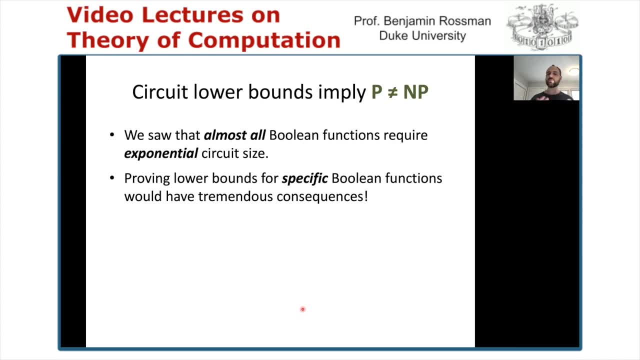 P from NP. So we saw that almost all Boolean functions require exponential size circuits. But proving lower bounds for any specific Boolean function would have great consequences. And just to restate what we just observed, if any language in NP, for instance, satisfiability, in fact 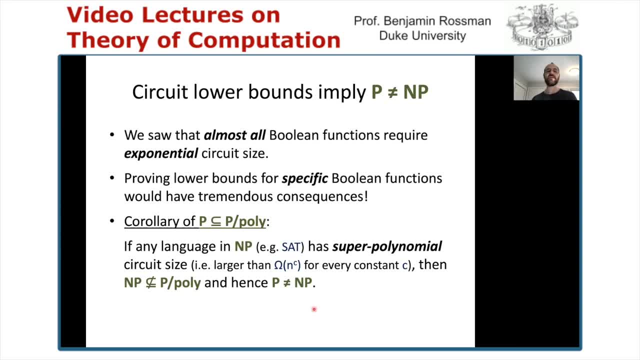 without loss of generality, you could consider any NP-complete problem. So if any language in NP has super-polynomial circuit size so larger than omega n to the c for every constant c, well that shows that NP is not contained in P slash poly. 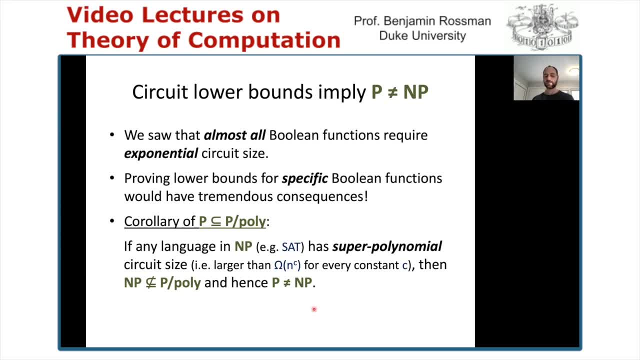 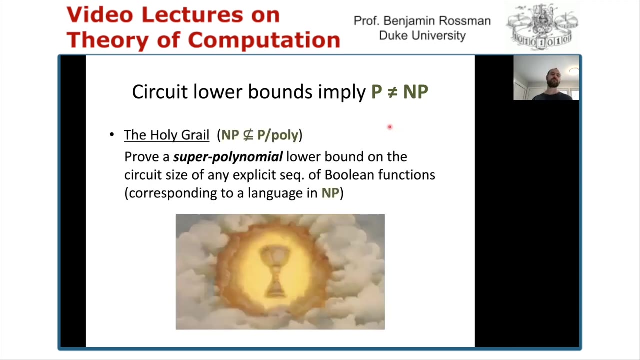 and therefore P not equal to NP. So this is one of the reasons to study circuit complexity is that Is that it provides a combinatorial version of this P versus NP problem, And we can hope to study these important questions from that perspective. 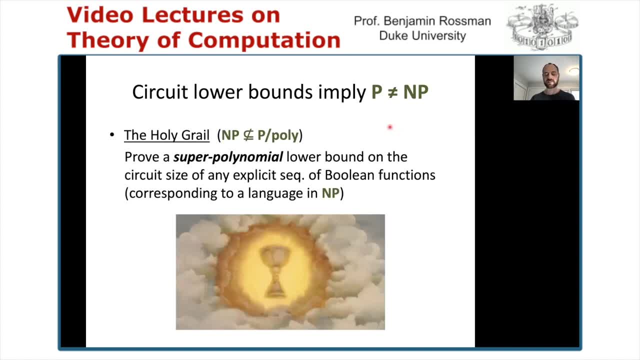 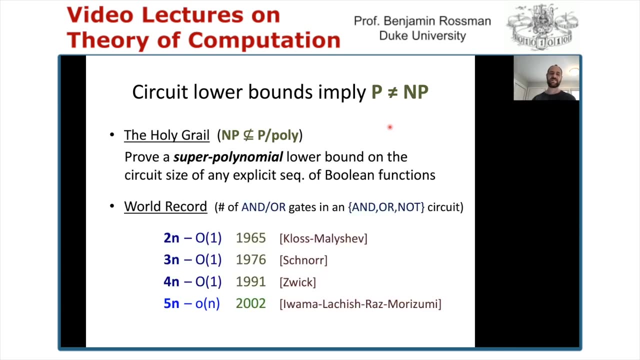 And so this is, as I said, the holy grail of circuit complexity, to prove a super-polynomial lower bound on the circuit size of any explicit sequence of Boolean functions. So Yeah, Unfortunately, proving lower bounds is hard, And this is illustrated, I think. 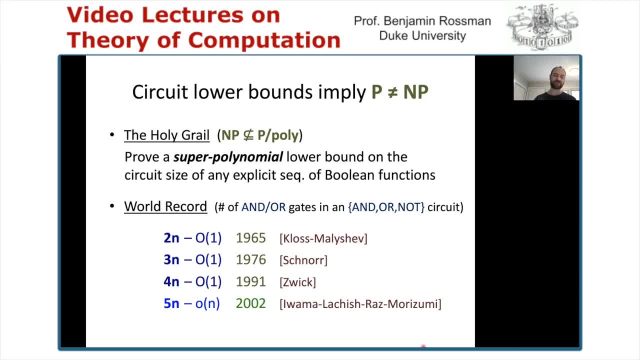 by considering the sequence of world records of the strongest known lower bounds for explicit Boolean functions, here measured in terms of the number of AND and OR gates in Boolean circuits- And as you can see, progress on lower bounds has been very, very slow. 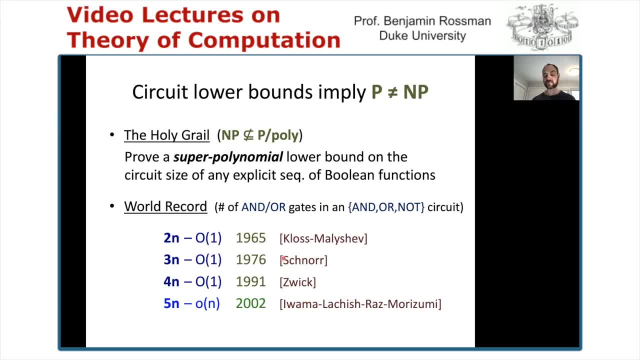 And currently the strongest Lower bound known is just shy of 5N. So we have merely linear lower bounds, whereas we need a super-polynomial lower bound to resolve big open questions. People have also considered circuits in the so-called full binary basis. 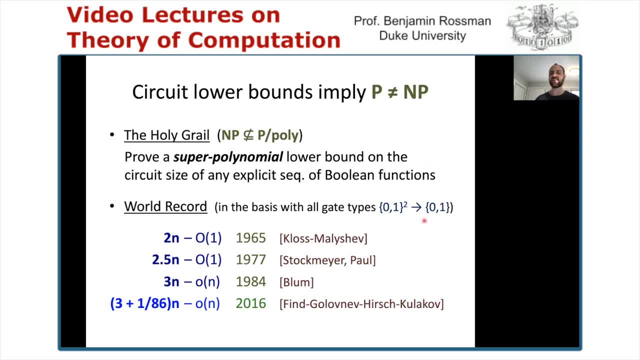 So if we allow all binary Boolean functions as gates in a circuit, this is a more powerful model than just Boolean circuits. So the lower bounds are even weaker And, as you can see, progress is similarly slow. There was recently, in fact, a breakthrough. 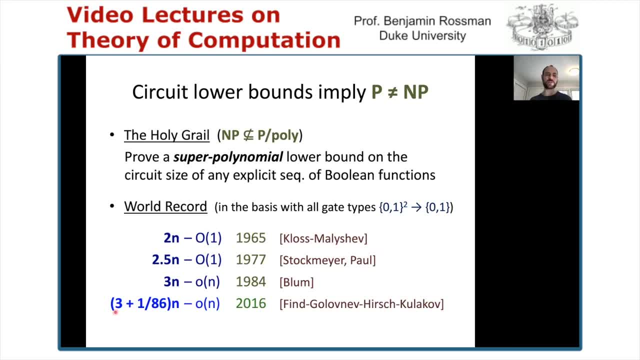 in proving long-standing 3N lower bound to 3 plus 1 over 86.. But I think this well illustrates the challenge of proving circuit lower bounds. So next I wanted to say something about the technique that's used to prove these lower bounds. 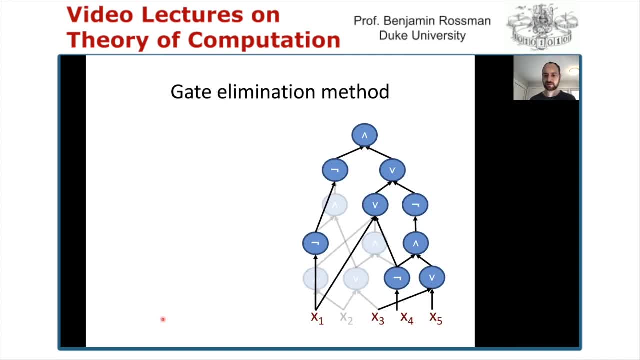 This is known as the gate elimination method. OK, And the idea is pretty simple. So we want to prove a lower bound on circuit size, So let's say a linear lower bound of the form C times N for some constant C. So suppose we could do the following: 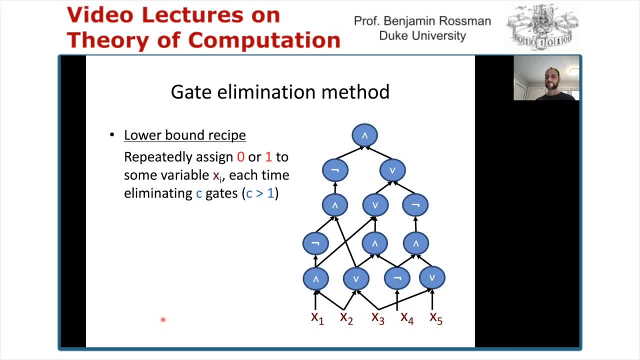 We could repeatedly pick some variable xi and assign it to either 0 or 1 in a way that again eliminates at least C gates from our circuit each time we do this. So let me illustrate what I mean. So here, consider the variable x2.. 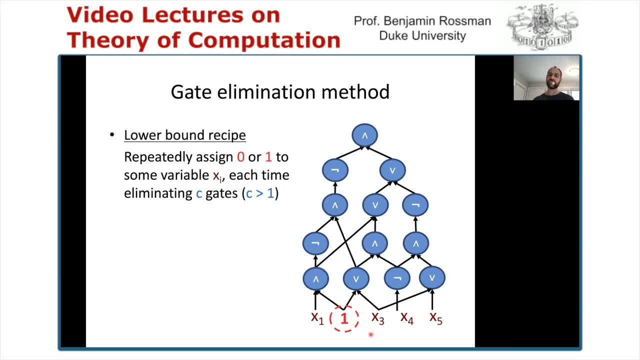 And suppose we substitute 1 for x2.. And let's see how this simplifies the circuit. So consider this AND gate. We have a 1 feeding into an AND gate, But this means that the gate only depends, therefore, on its other arguments. 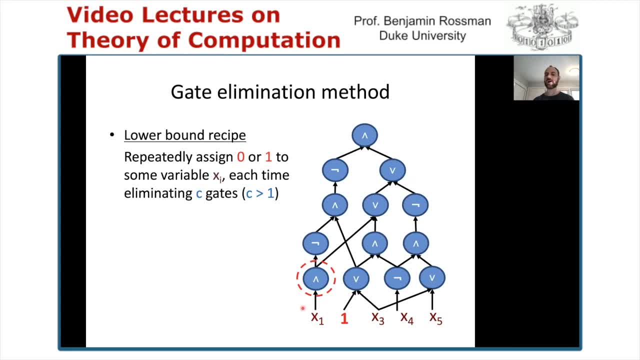 So this lets us eliminate this wire. And now we have this OR gate. So we have a 1 feeding into an OR gate. So that means that the OR gate will produce the value 1, no matter what its other argument is. 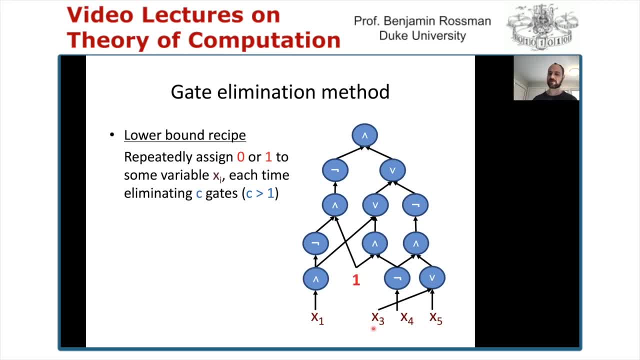 So we can eliminate that gate and propagate this 1.. And now we have a 1 feeding into 2 AND gates. So, as we saw, we can eliminate those wires And we can perform For additional simplifications. we have these three gates here which receive only one wire. 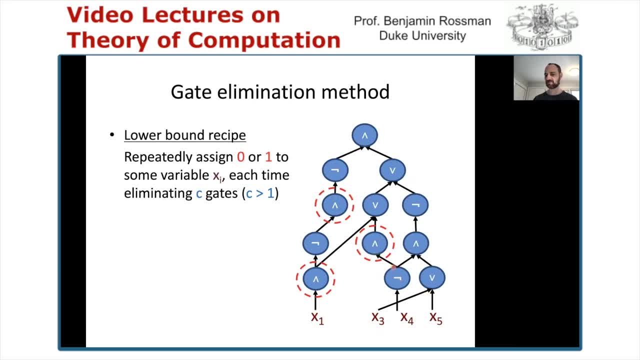 So this means that we can bypass those gates and just put wires directly, like this. We could even notice now we have two negation gates And therefore they cancel each other. So just by some local simplification process, we've reduced our circuit to this form. 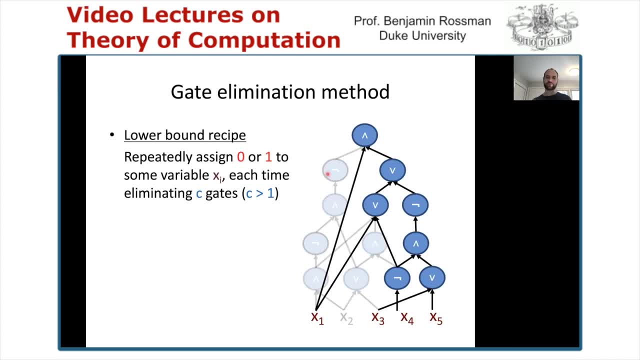 And so, here you can see, the gates are eliminated. So in this case we've eliminated six gates And right. So, assuming you could do this, eliminate at least c gates for at least a constant fraction of the time. this would give you some bound, lower bound, say cn. 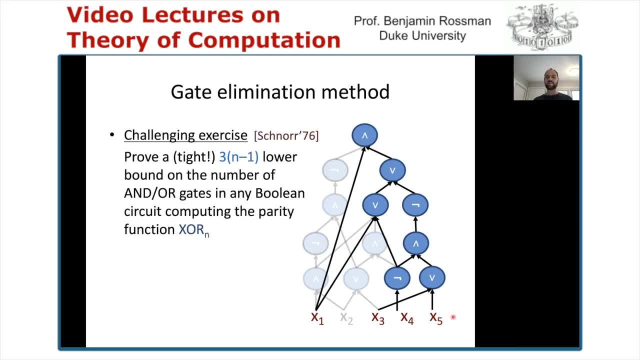 if you could always do this, And I'll leave it as an exercise to show that, using this exact method, you can Prove a tight lower bound of 3n minus 3 on the number of and and or gates in any Boolean circuit. 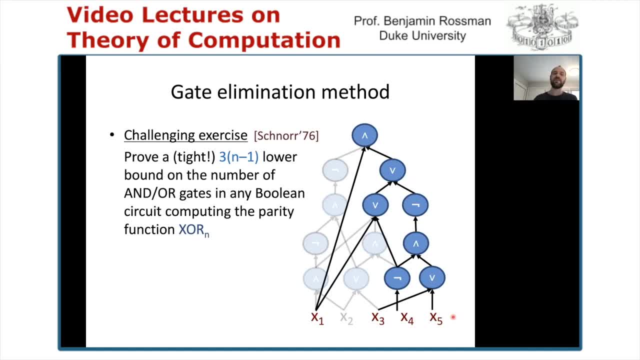 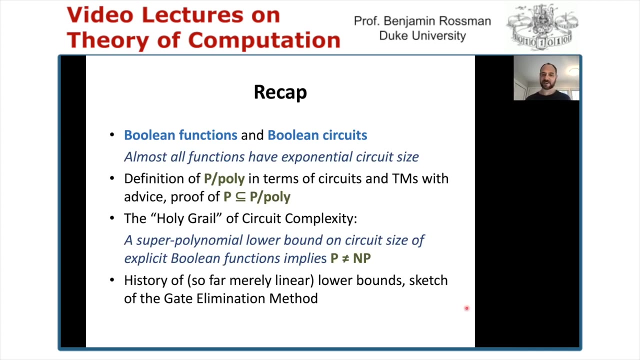 computing the parity function. So we already saw earlier that this 3n minus 3 is an upper bound, And you can prove that this is exactly tight using this simple argument. So this is the gate elimination technique And Let's- yeah, let's- recap what we've seen so far. 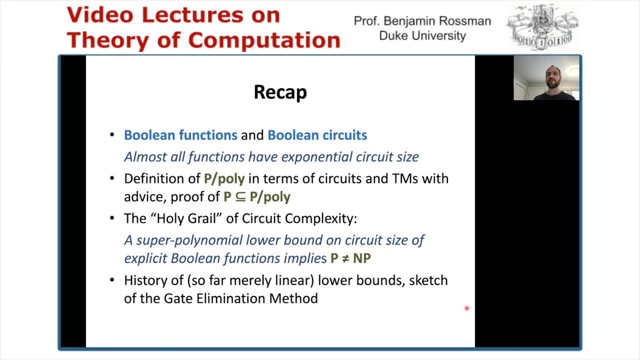 So we've defined Boolean functions and Boolean circuits And we prove Shannon's theorem that almost all Boolean functions require exponential circuit size. We've defined the class p slash poly both in terms of Turing machines circuits and in terms of Turing machines with advice. 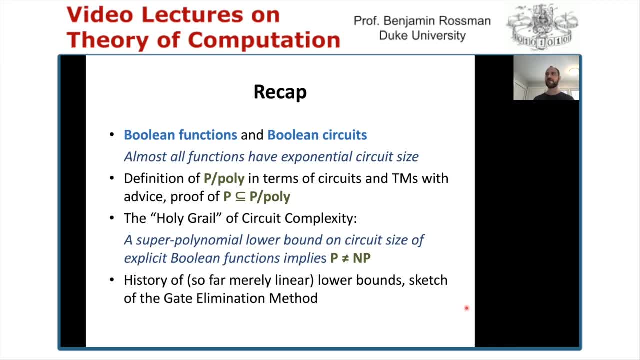 And we've given a proof that p is contained in p slash poly via this quadratic simulation of Turing machines by circuits. And we discussed the holy grail of circuit complexity, which is to prove a super polynomial lower bound on the circuit size of explicit Boolean functions. 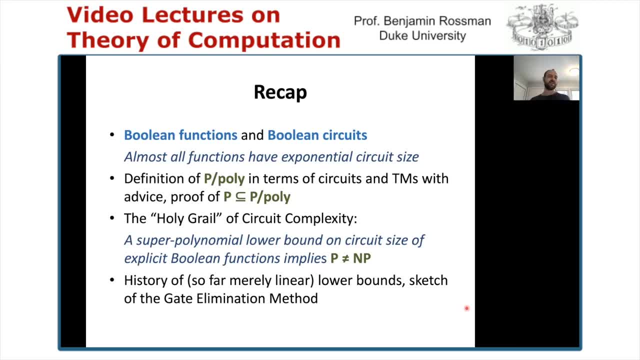 And this would imply p not equal to np. And we had a look at the history of lower bounds known to date, So far merely linear, And we gave a sketch of a gate elimination method which can be used to prove some of these lower bounds. 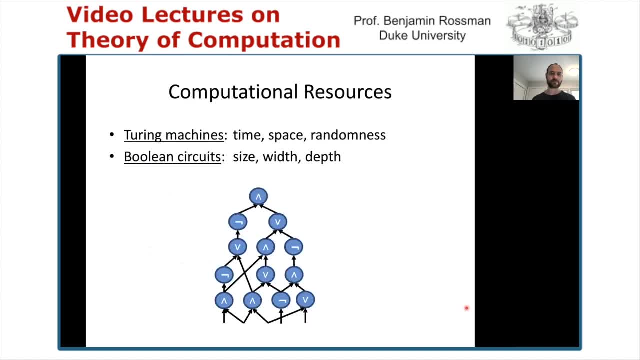 So next let's have a look at some of the other computational resources of Turing machines on the one hand and circuits on the other hand. So in the setting of Turing machines we study time complexity, space complexity, randomness, And for Boolean circuits we've already discussed size. 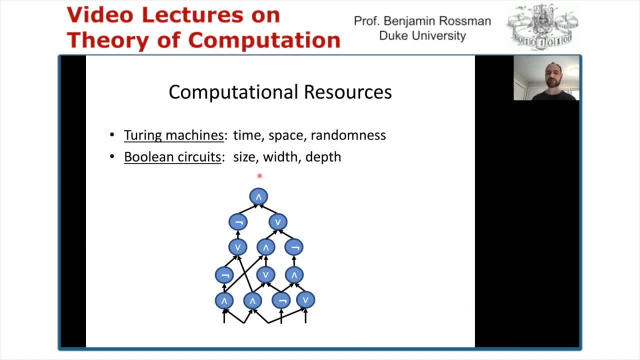 We defined but haven't yet discussed depth as a resource You could also look at- Let's see- Width of Boolean circuits. So if we have a Boolean circuit where the gates are arranged in layers, with wires going from one layer to the next, 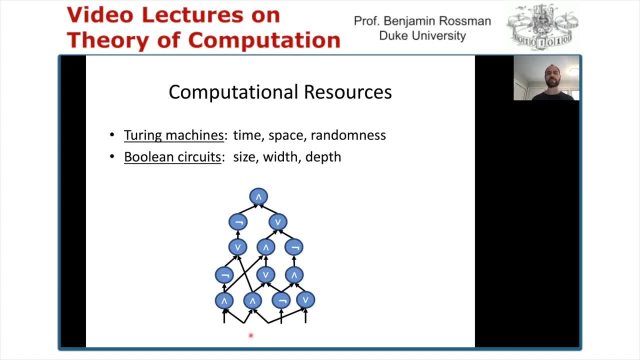 then the width would be the maximum number of gates on any layer. And we saw that time complexity on Turing machines corresponds to circuit size. So space complexity turns out to correspond in a similar way to circuit width And analogous to that, Analogous to the definition of P slash poly. 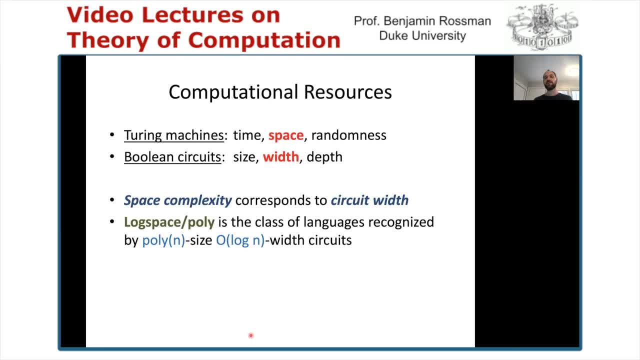 there's the class log space slash poly, And this turns out to be equivalent to the class of languages recognized by polynomial size. log width circuits- Just to mention many of the classes we study in circuit complexity- turn out to have equivalent characterizations. many 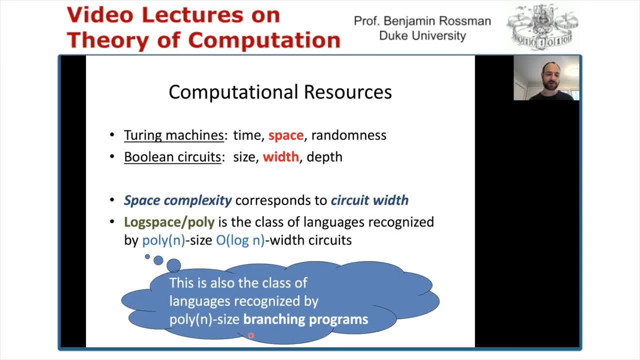 different equivalent characterizations. In the case of log space slash poly. this is also the class of languages recognized by polynomial size branching programs. So I'm not going to define branching programs, but if you've seen decision trees before, then branching programs are like a circuit version. 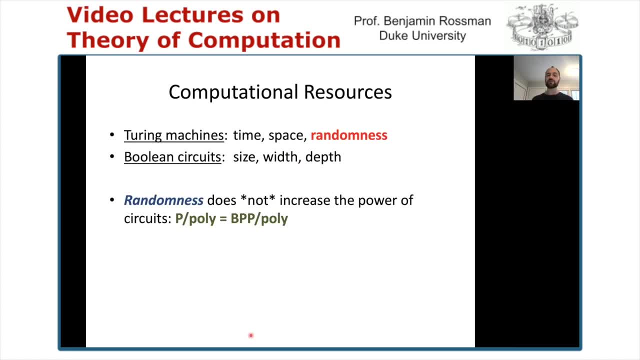 of decision trees. So randomness is an interesting resource in the setting of Turing machines. in the setting of uniform complexity theory. It turns out that in the setting of non-uniform Boolean randomness does not increase their power. So you can show that P slash poly equals BPP slash poly. 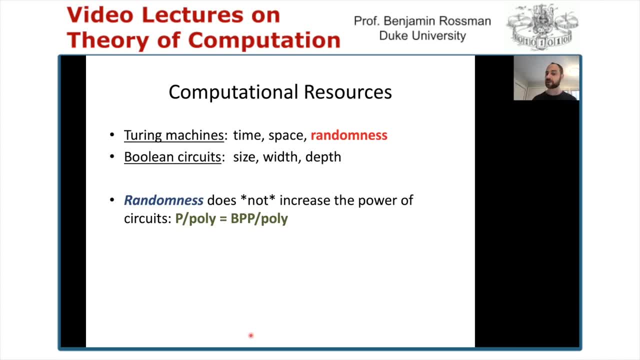 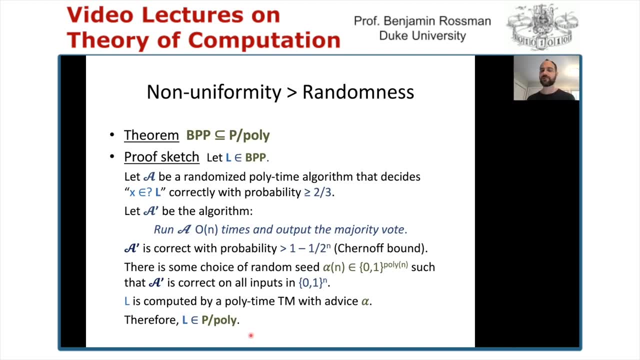 So in the non-uniform setting, And I'll give a very quick sketch of how the proof of that result goes. So let's just show that uniform BPP, the class that you've encountered so far, so randomized poly time algorithms, is contained in P slash poly. 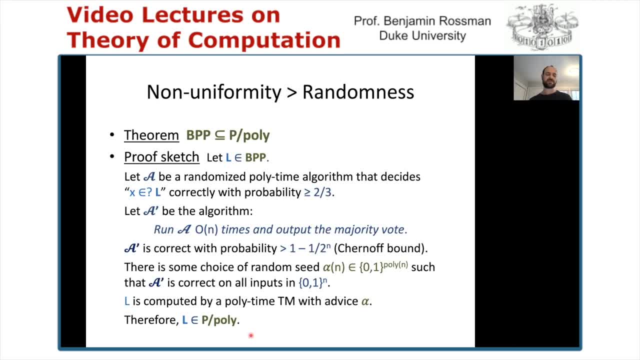 Poly sized circuits. So you can also think of this result as saying that non-uniformity is more powerful than randomness. So here's a sketch of the proof. So consider a language: L in the class BPP. So this means that there exists a randomized poly time. 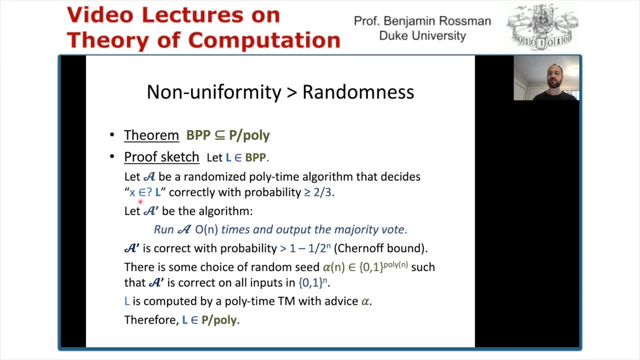 algorithm A that decides membership in L And it gives the correct output with probability at least 2 thirds. So that's the proof for any x. So now we're going to define another poly time algorithm, A prime, which is simply to run the algorithm A. some order. 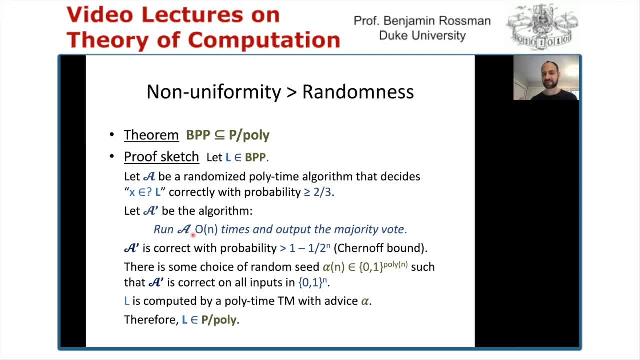 n times and output the majority answer. So output the majority answer And one can easily show using the Chernoff bound that A prime is correct with probability at least 1 minus 1 over 2 to the n. So we can take some error 1. third. 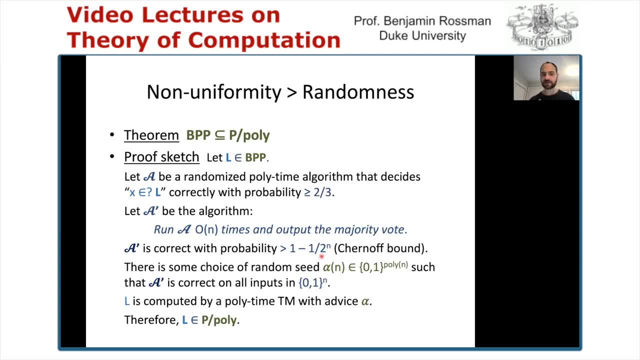 And we can reduce it all the way down to exponentially small error by just repeating the randomized experiment some order n times, with independent randomness each time. So this is still a poly time randomized algorithm, And now, By the magic of the probabilistic method, 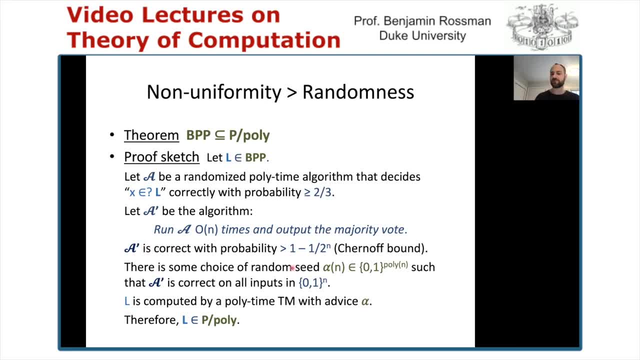 it follows that there exists some choice of the random seed for this algorithm, A prime, such that A prime is correct on all inputs. So because the number of inputs is 2 to the n and we've reduced the error probability down to below 1, 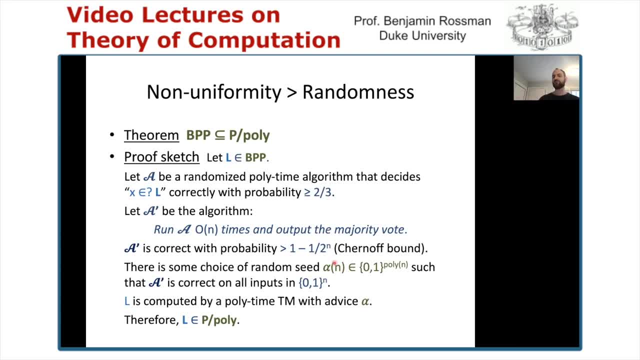 over 2 to the n. it follows that there's some choice of the random seed for which this algorithm is correct on all inputs of length, Then great. So now it follows immediately that this L is therefore computable by a polynomial time Turing machine. 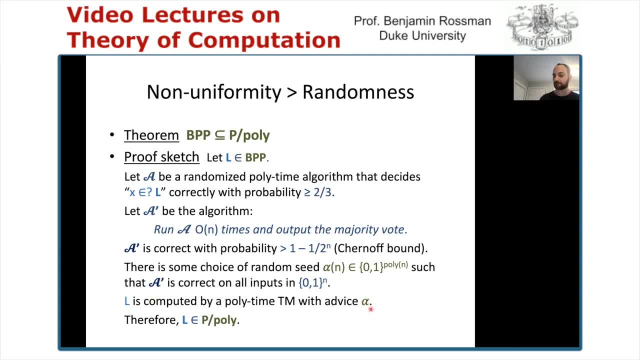 with this advice string alpha, You just simply run A prime with alpha playing the role of the randomness And therefore by our characterization of P slash poly in terms of poly time Turing machines with advice, this shows that L is in P slash poly. 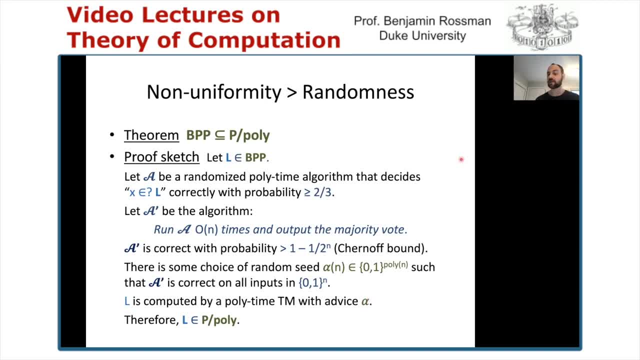 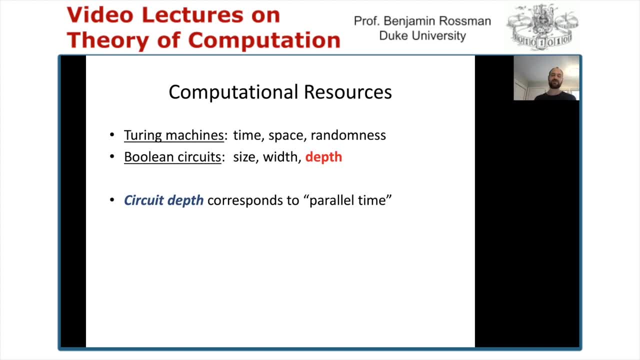 OK, So this is the proof that non-uniformity is more powerful than randomness. So, finally, we come to a very interesting resource of Boolean circuits, which is the depth. So recall that the depth of the circuit is the length of the longest path from an input to the output. 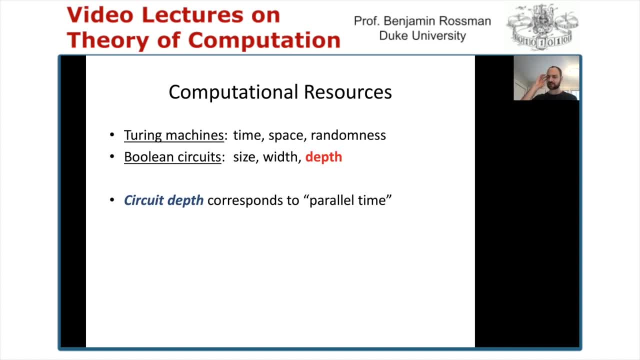 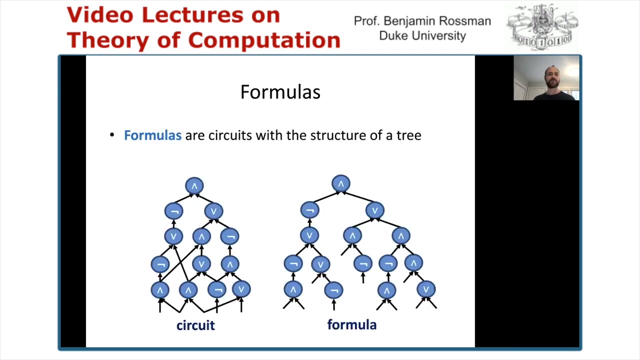 gate And this. This measure corresponds to parallel time, So corresponds to time for parallel algorithms with multiple processors. But it's also tightly connected to another complexity measure called formula size. So let me now define for you what are formulas. So formulas are simply circuits, Boolean circuits. 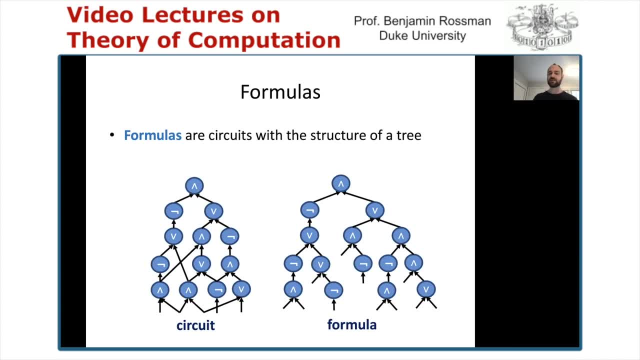 with the structure of a tree. OK, Meaning each gate has, or each node in the formula has out degree 1.. OK, So this means that it will have the structure of a tree, Whereas in a general circuit you can have a gate which feeds its result to multiple gates. 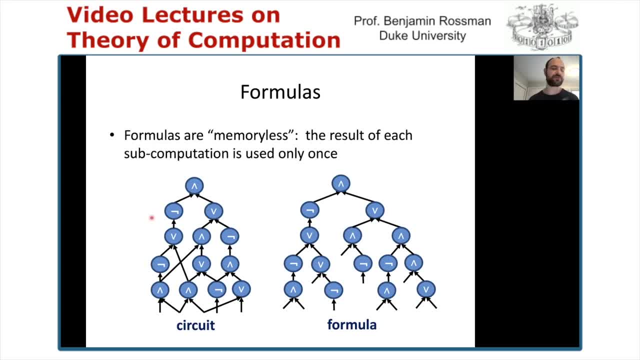 above it, And you can think of formulas as being a memoryless model of computation, in the sense that the result of each sub-computation gets used only once. So each gate only feeds its answer to one gate above it. OK, And intuitively, this should mean that formulas 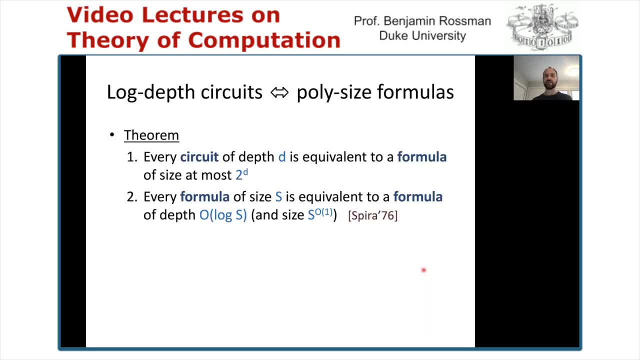 are a weak model of computation. So this correspondence between circuit depth and formula size is made concrete by the following theorem. So first, every circuit of depth d is equivalent to a formula of size at most 2 to the d. OK, We'll see the proof of this in a moment. 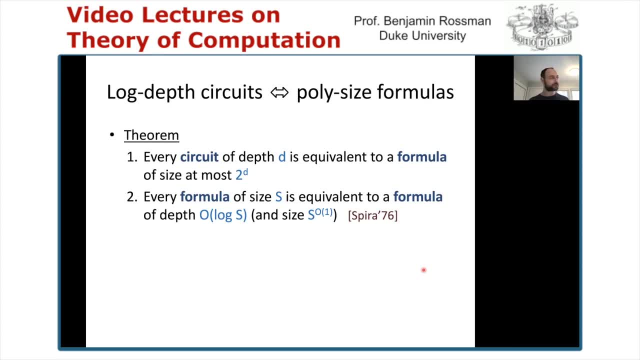 And then the more interesting direction. every formula of size, s, is equivalent to a formula of depth order log s. OK, And therefore by part 1, the size will be s, 2 to the order of log s, so s to some constant. 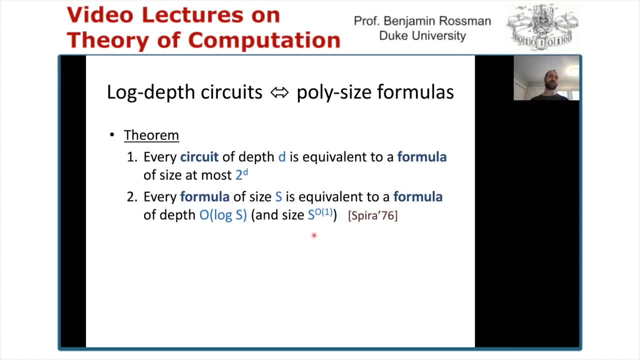 OK, So in other words, this is saying that with a polynomial blow-up in size, we can balance a formula so that it has depth, which is just logarithmic. OK, And I'm going to illustrate the proof, sort of give a proof by picture of both parts of this theorem. 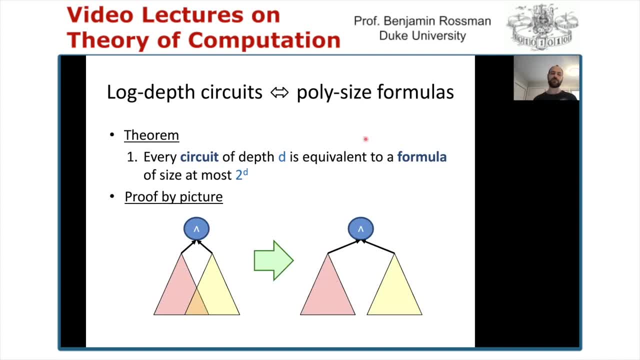 So for part 1, well, we're just going to convert a circuit to a formula in the obvious way. So for each gate in the circuit, if it has takes two subcircuits that feed into it, we just make disjoint copies of those subcircuits. 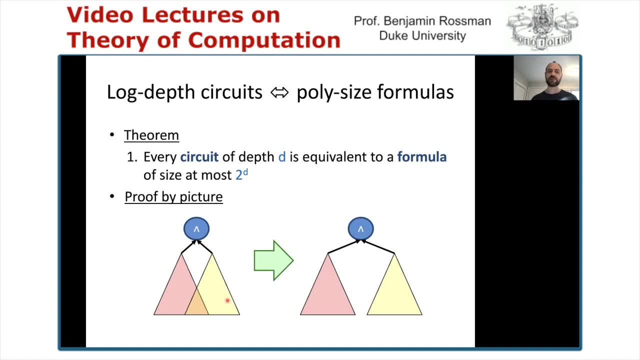 And then we repeat this process. So, start at the root, Starting at the root, We do this And then repeat this process inside of the red triangle and the yellow subcircuit, OK, And you do this all the way down And it's easy to show that the formula size that you get. 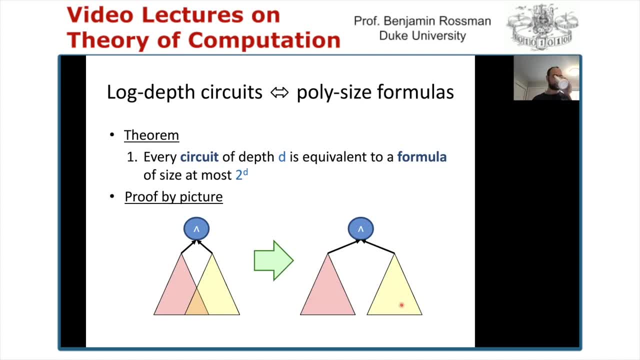 is at most 2 to the d. OK, So for the other direction, we're going to start off with a formula of size s And we're going to show how we can convert it to a formula of depth order log s. So here, consider this orange formula of size s. 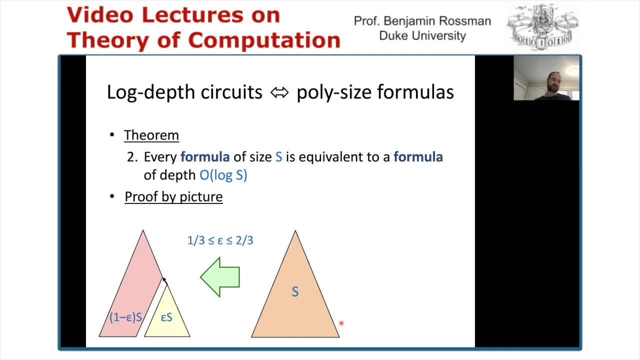 So the first step is to we're going to split this formula. We're going to find some edge, some wire that is in this formula. If you remove that wire, you'd split the formula into two subformulas, each of size between 1- 3rd s and 2- 3rd. 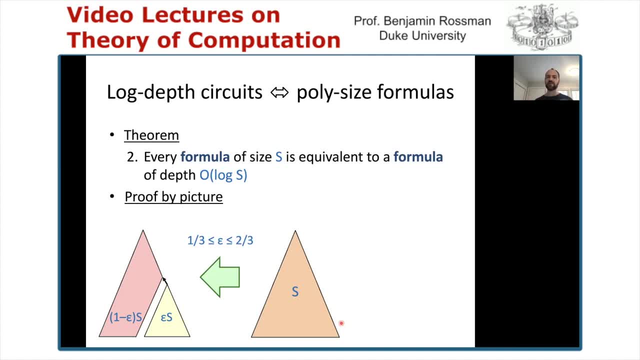 s. So the claim is, in other words, that there exists some subformula of depth order log s, There exists some subformula of the orange formula whose size is between 1, 3rd and 2, 3rd s, And to see this it's very easy. 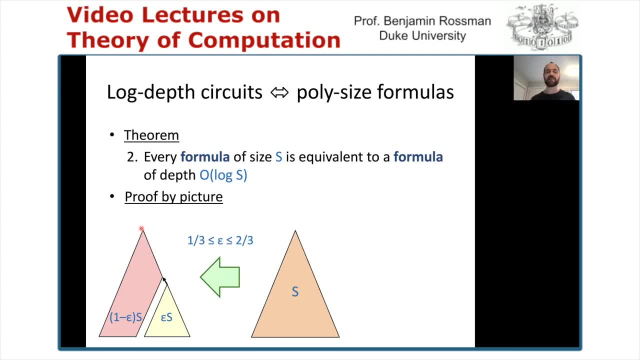 So a formula, after all, is a binary tree, a rooted binary tree. So start at the top And consider a walk down the formula where at each point you descend to the larger of the two subformulas below you And the claim is that, well, at some point. 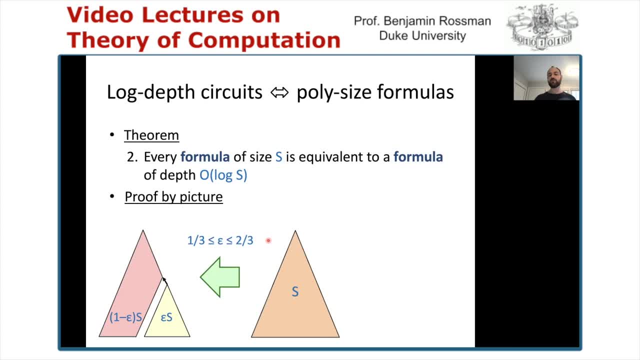 we have to reach a subformula of size between 1- 3rd s and 2- 3rd s, And this is simply because each time we descend, we're reducing the size by at least 1 half And therefore it's impossible to pass from size above 2- 3rd. 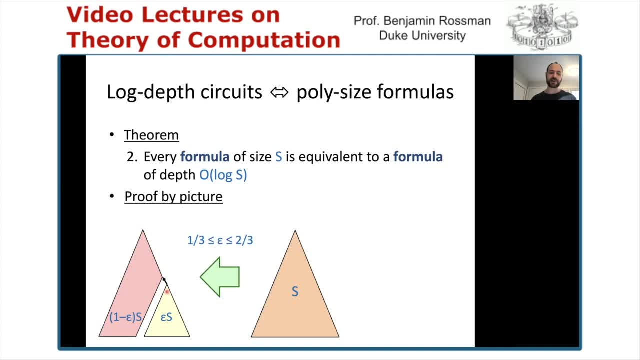 s to below 1 3rd s. So we find such a subformula, Subformula like this, And then we do the following transformation. Consider the following formula: What I've done here is I've taken two copies of the yellow subformula. 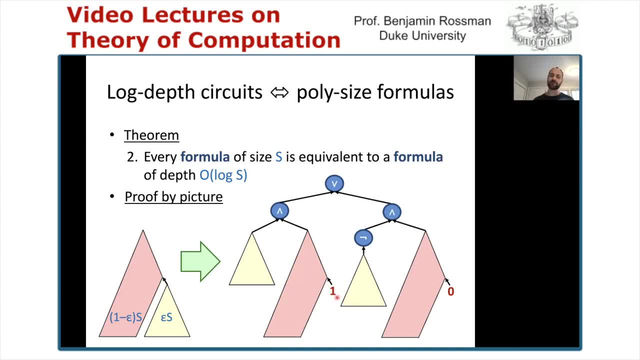 and then two copies of the red subformula, where here I'm substituting 1 for the yellow subformula and here I'm substituting 0. And I claim that this formula on the right it computes, It's the same Boolean function as the formula on the left. 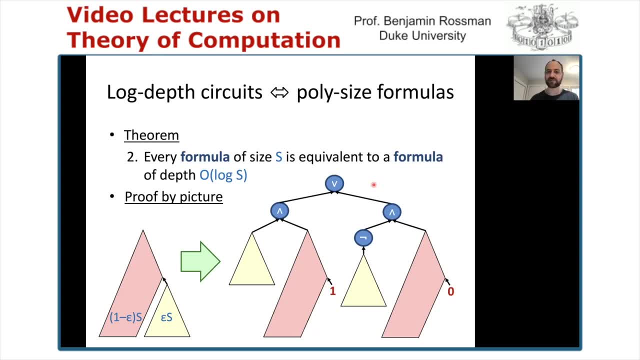 And so this is easy to see if we just verbalize what is this formula doing. It's saying: either the yellow subformula evaluates to 1 and this red subformula with 1 substituted evaluates to 1.. Or the yellow subformula evaluates to 0. 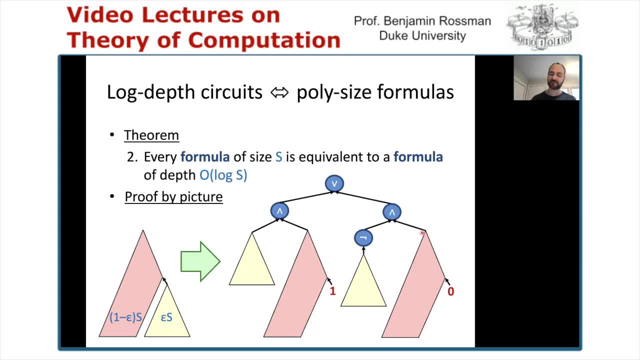 and the red subformula with 0 substituted, evaluates to 1.. Right, So this equals 1 if, and only if, this guy equals 1.. OK, And then. so we've transformed this. We started off with this orange formula and we've transformed it so it has this form. 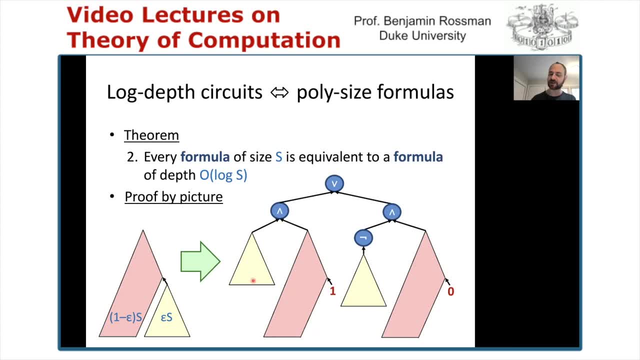 And then we're going to recurse. We're just going to do the same balancing process in each of these four subformulas And since each of these four subformulas has size- at most 2, 3rds s- Cephas, Stormi-, This means that this recursion only has depth order log s. And when you think about the resulting formula, This means that the note that we're increasing the depth by by just three each time, Right? So the final formula we get in this way will have depth order log s. 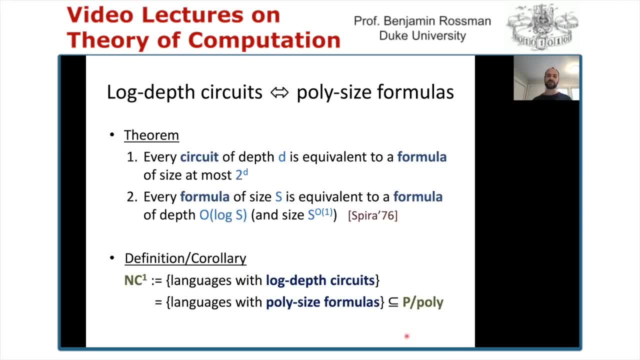 Cephas Stormi- Okay, so that's. this is the the, the term we just showed, And this leads to the following definite definition: slash corollary: Cephas Stormi- So the class, the complexity class of languages decidable by log depth circuits, the circuits of depth order, log n. This is known as NC one. 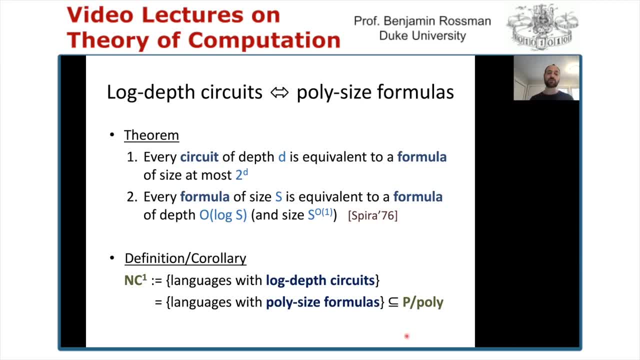 Cephas- Stormi- And, as a corollary of the theorem, This class is equivalent to languages with a depth order log n- Cephas- Stormi- And, as a corollary of the theorem, This class is equivalent to languages with poly size formulas. 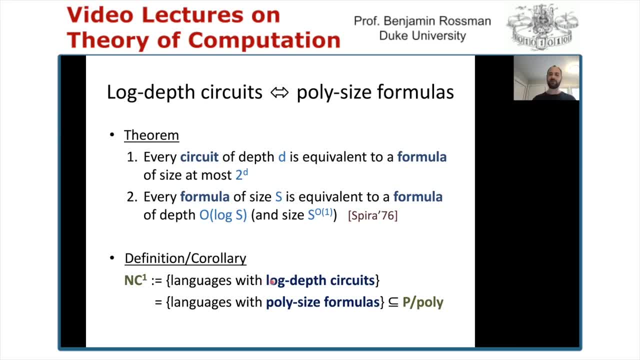 Cephas Stormi- Right, so to see why. So every log depth circuit is equivalent to a poly size formula by part one- Cephas Stormi- And every poly size formula is equivalent to a log depth formula by part two. and every depth, two formulas, Sorry. And since formulas are our circuits, this shows that poly size formulas are equivalent to log depth circuit. 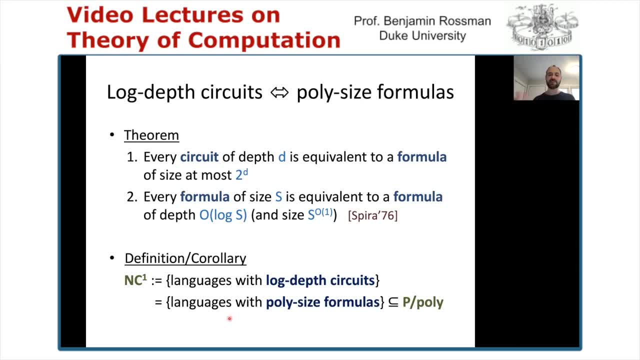 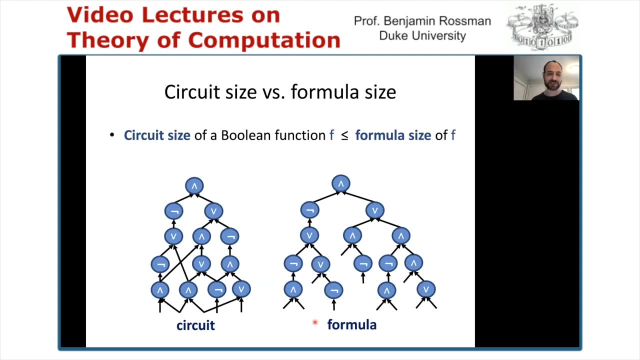 Cephas Stormi- And, moreover, follows that this class, and see one, is a subclass of P slash poly- Cephas Stormi- Because poly size formulas are subclass of poly size circuits- Cephas Stormi-. Okay, so now we have these two different size notions for Boolean functions. we have circuit size and formula size and clearly circuit size of a Boolean function is at most the minimum formula size. 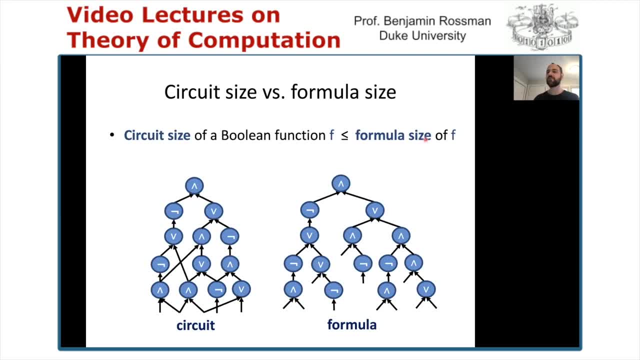 Cephas Stormi- Right, because Cephas Stormi- The smallest formula for F is also a circuit, so that that provides an upper bound on the smallest circuit size of F. Cephas Stormi- So therefore, I mean it follows that proving lower bounds for formulas is necessarily an easier task than than for circuits. So we saw that proving circuit lower bounds is hard. The best lower bounds that are known are merely linear. What about formulas? 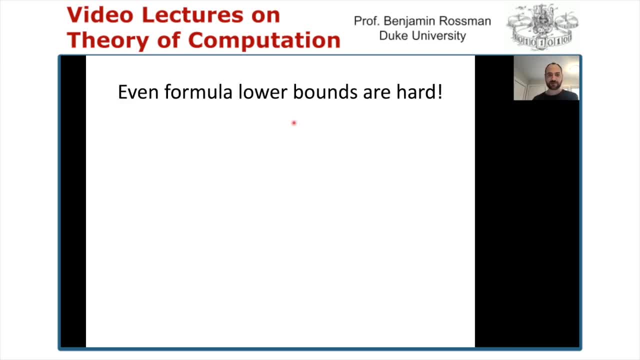 Cephas Stormi- So it turns out that even formula lower bounds are hard. And here here's the history of the strongest known formula size lower bounds for explicit Boolean functions: Cephas Stormi- So this is a. this problem has been studied for a long time And there's, you know, there was a very gradual sequence of improvements, but for over 20 years the strongest lower bounds have been stuck at just shy of cubic. 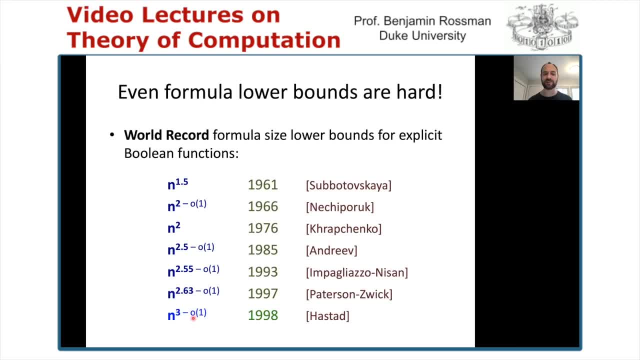 Cephas Stormi- So there was recently Cephas Stormi- Some low order improvement inside of this little old one by Abishai Tal a few years ago. but this is one of the major frontiers and complexity theory to prove lower bounds better than better than n cubed. 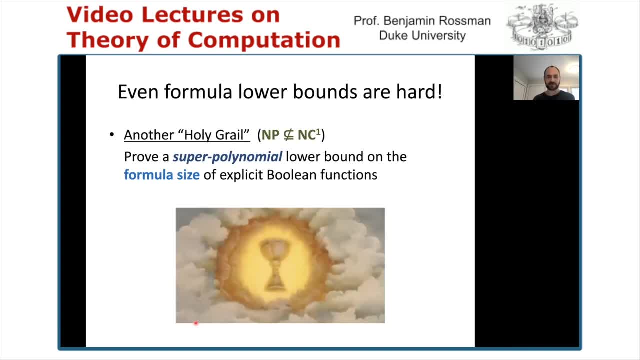 Cephas Stormi- And this is also another holy grail problem in circuit complexity: to prove a super polynomial lower bound on the formula size of explicit Boolean functions: Cephas Stormi- And as we saw. So this this would show that. 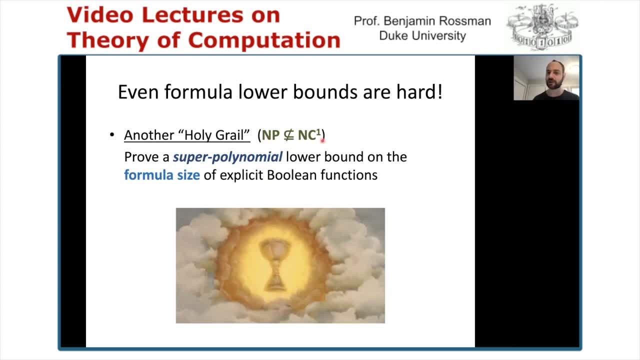 Cephas Stormi- This would show that NP is not contained in the class and see one: Okay, so this is a would be a weaker result than NP, not in not contained in P slash Polly, but something which necessarily, we would need to show first. 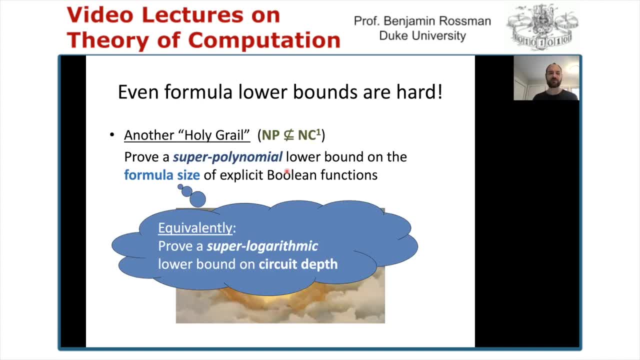 Cephas Stormi- And right, and and. as a consequence of the theorem We just saw, this is equivalent to showing a super logarithmic lower bound on circuit depth- Cephas Stormi- So a lower bound better than Cephas Stormi- C log n for any constancy. 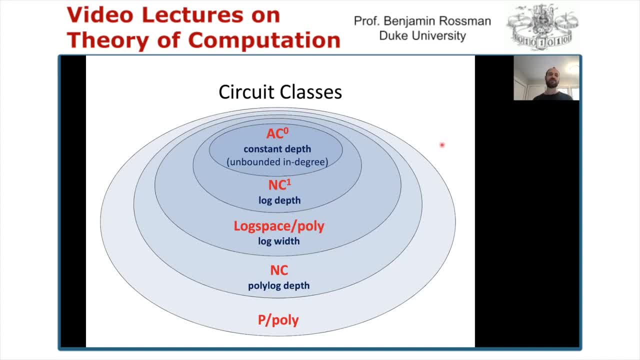 Cephas Stormi- So this is the last slide, Just to conclude. I wanted to mention some of the other Cephas Stormi- Complexity classes that are studied in circuit complexity in the non uniform setting. So we've already discussed some of these. we have P slash, Polly, which is Polly size circuits, and see one is log depth circuits. 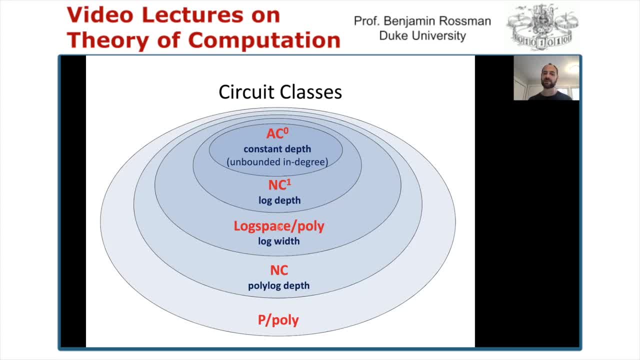 Cephas Stormi- Turns out that's contained in this class log space. Cephas Stormi- P slash Polly log with Polly size circuits- Cephas Stormi- And that's is contained in NC, which is Polly log depth circuits. and this is sort of the non uniform version of of efficient parallel algorithms, So algorithms running in Polly log time on polynomial many processes. 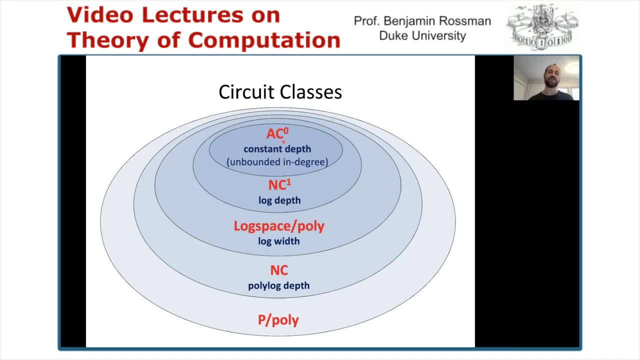 Cephas Stormi- And within and see one so very weak class that that's often studied as known as a C zero. Cephas Stormi- This is constant circuits where we allow and and or gates to have unbounded in degree. okay, and this is. 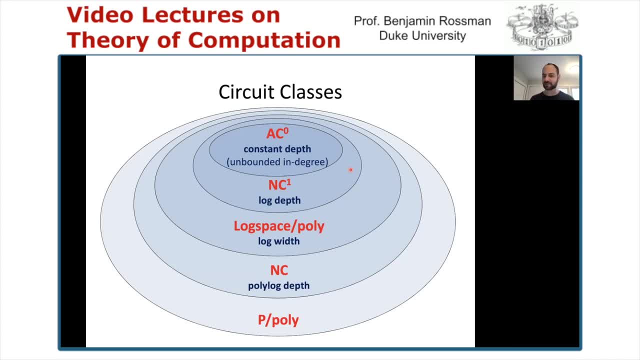 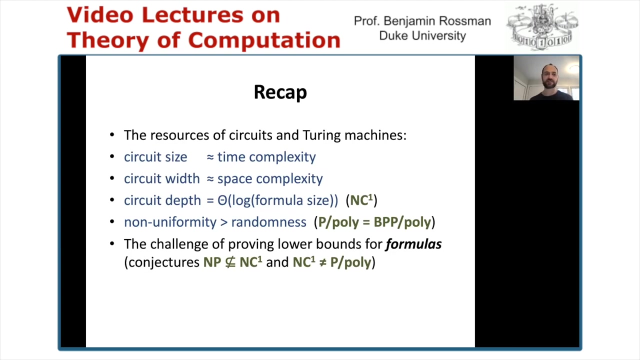 this class is sufficiently weak that there are techniques to prove strong lower bounds. in particular, it's known that the classic resultant circuit complexity shows that the parity function, which is computable in NC1, is not computable in AC0, and you can read more about ah. so yes, before giving the references, just to recap what we, what we showed in this last part. 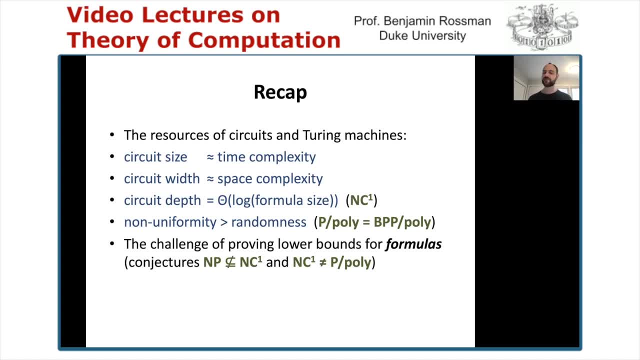 we discussed the different resources of circuits and Turing machines. right we we saw this connection between circuit size and time complexity. we mentioned that circuit width corresponds to space complexity and this notion of circuit depth we showed is is within a constant factor of log of formula size and this